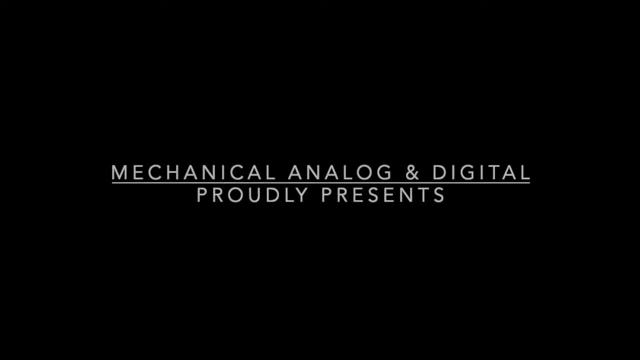 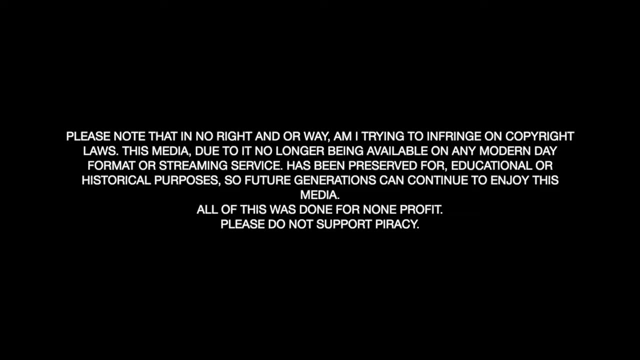 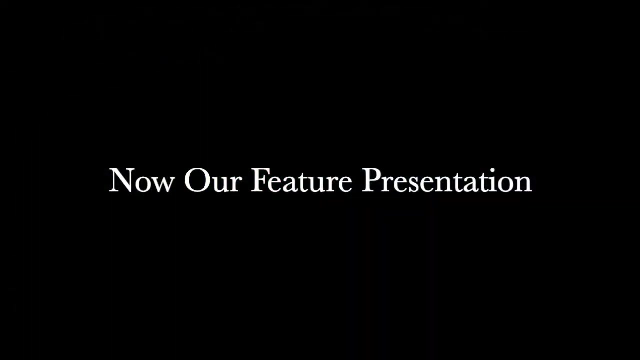 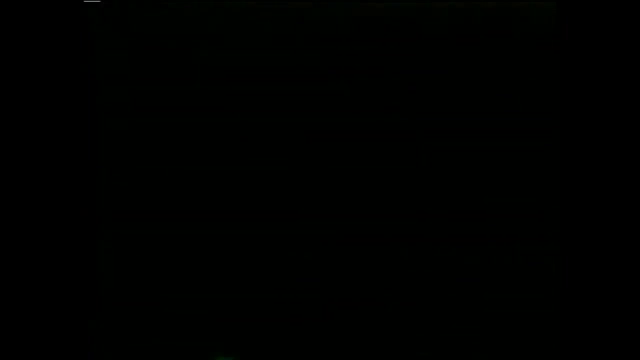 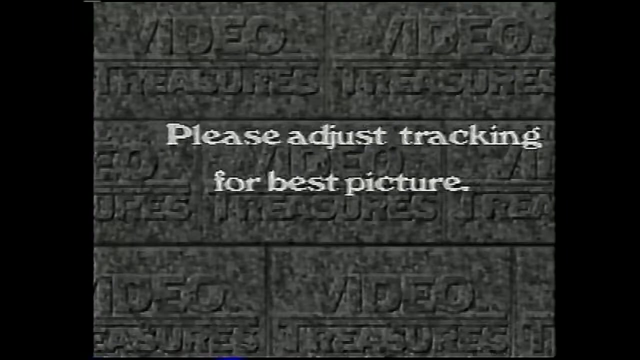 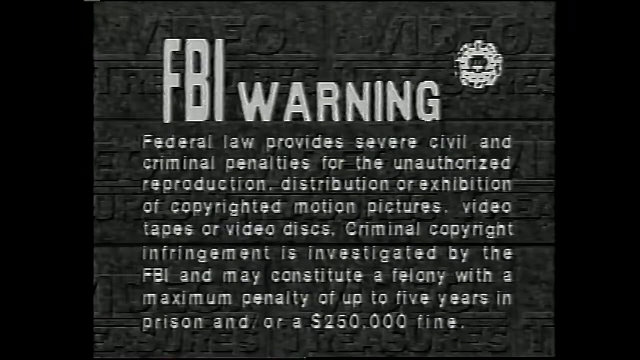 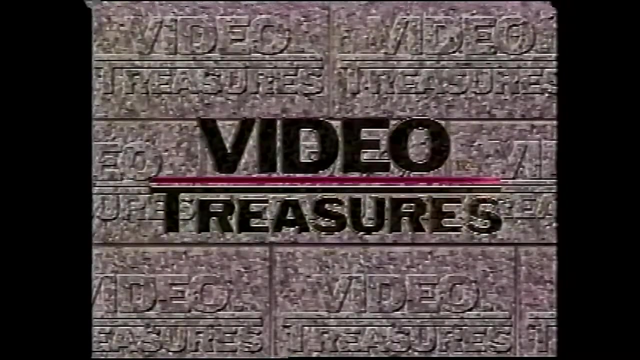 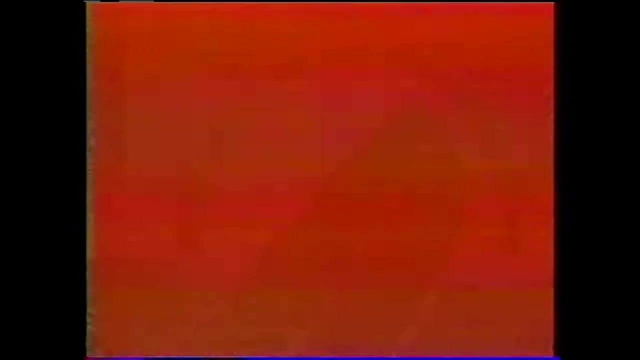 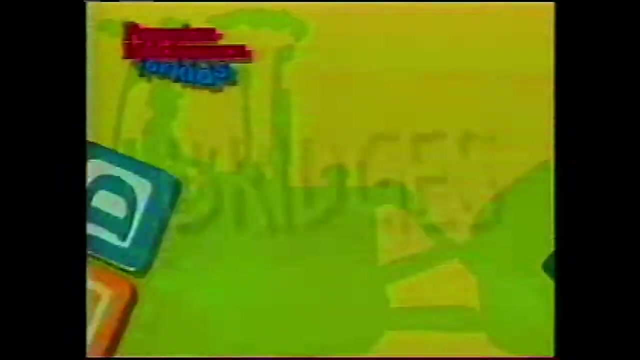 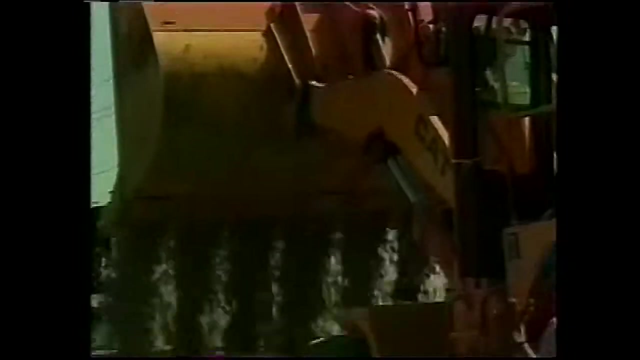 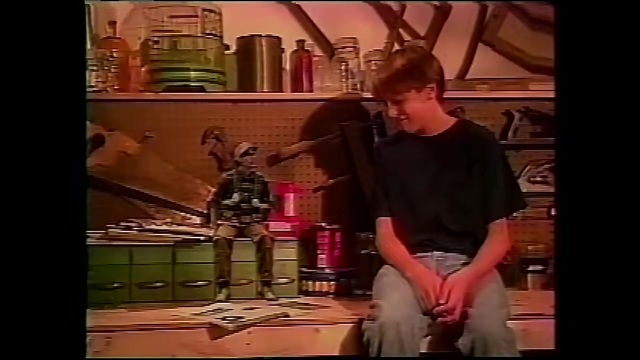 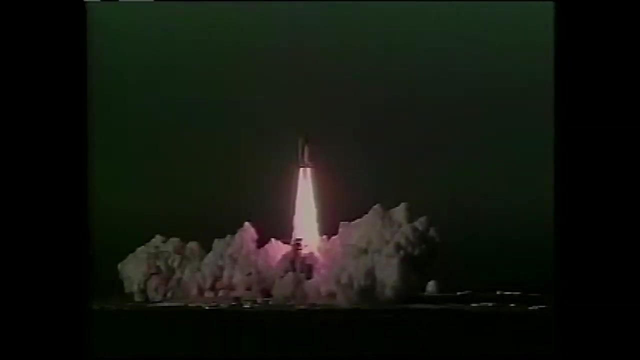 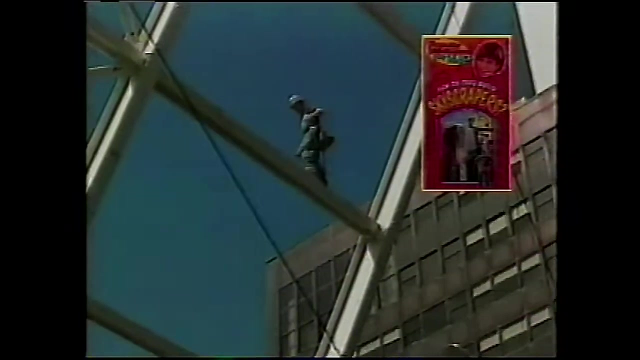 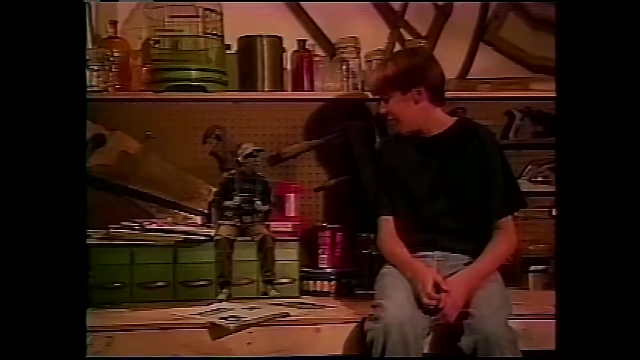 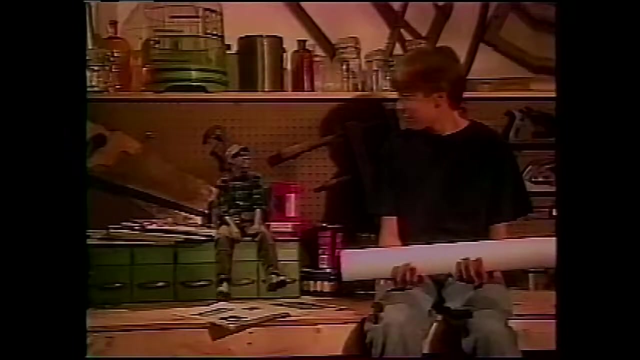 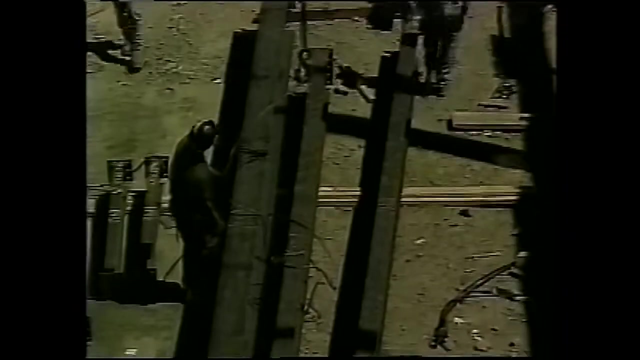 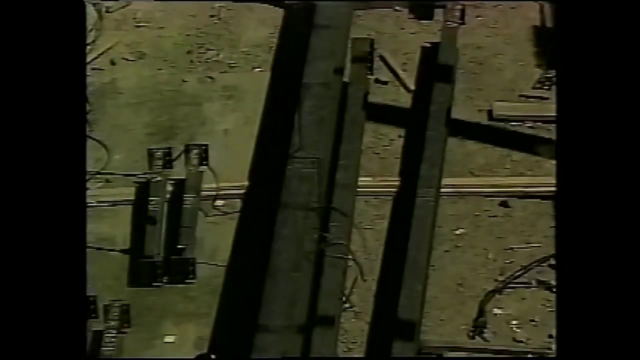 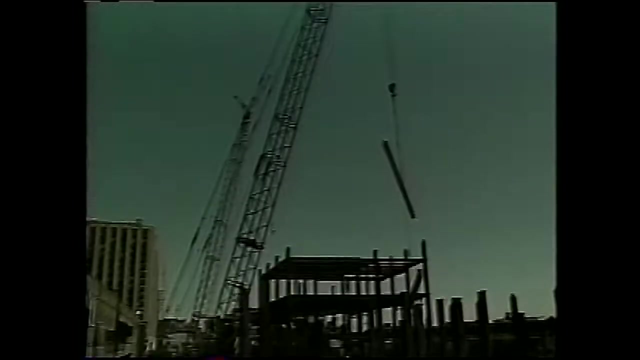 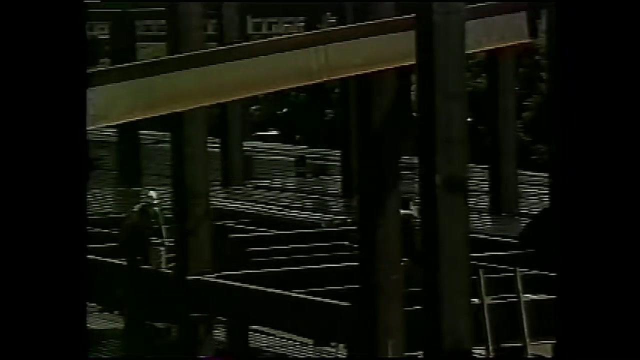 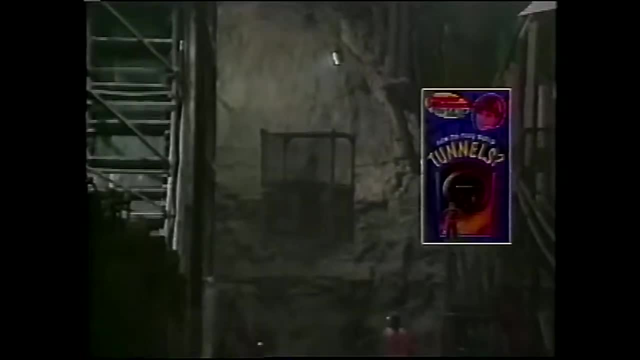 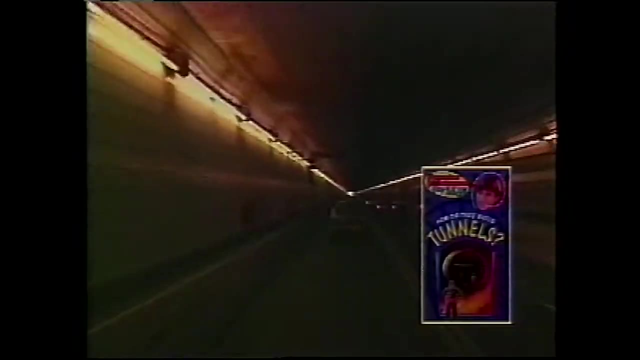 Ever wonder how they build tunnels? Well, now you can find out In How Do They Build Tunnels. you'll see giant drills boring through tons of rock and you'll learn how tunnels are built underwater After they dug a big trench in the bottom of the harbor. 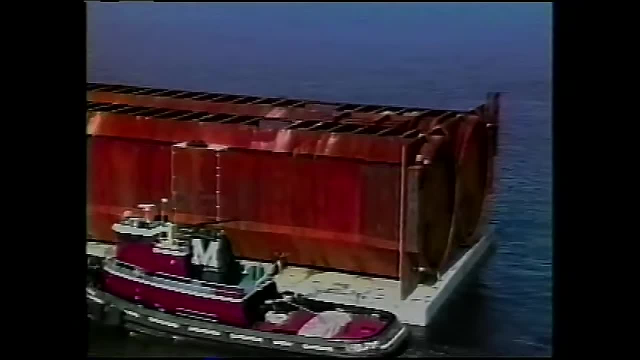 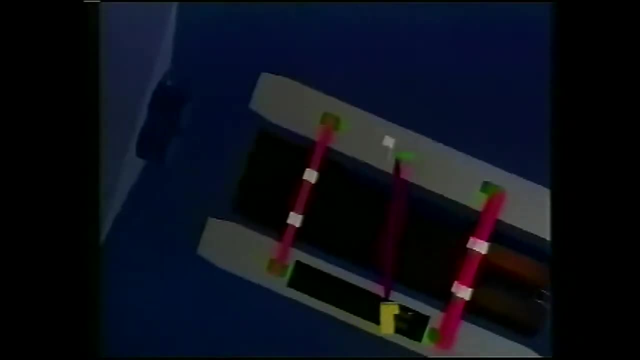 they brought the tubes out, two at a time, into the harbor on these barges. Check this aerial view out. See, this is a crane that lowers the sections into place. Well, it's just like a computer game. You're right, Mike. 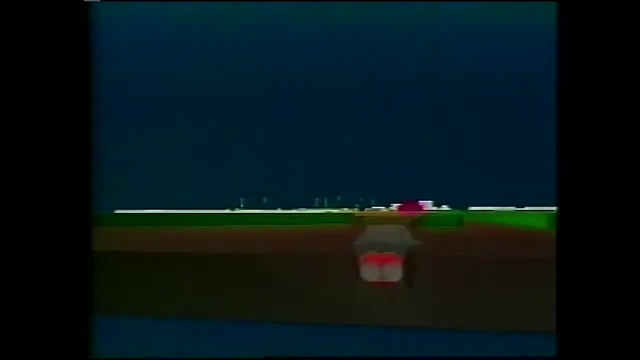 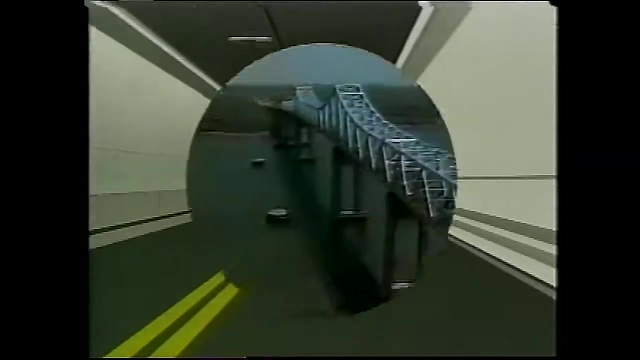 It's exactly the same kind of picture. Check this out. It looks like the back end of a jet engine. Is that what the inside of the tunnel will look like when it's done? Hey, you catch on quick. Think it's cool to drive over the water? 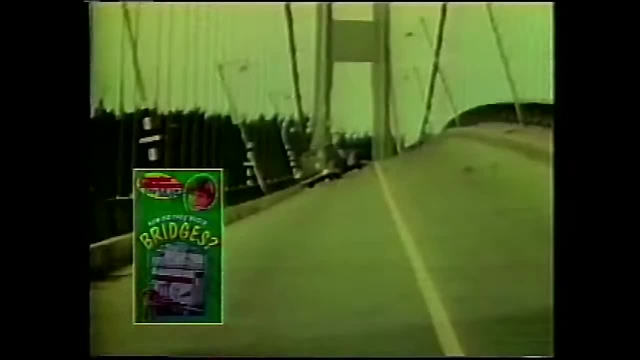 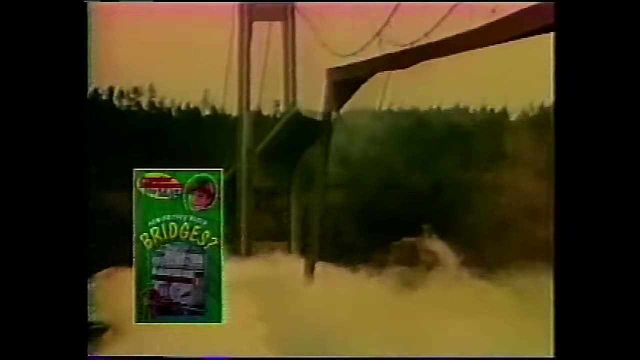 Then you'll want to check out How Do They Build Bridges. Yikes, Did anyone get hurt? Luckily no, But the builder of this bridge learned a big lesson about what wind can do to a suspension bridge. Hey kids, check this out. 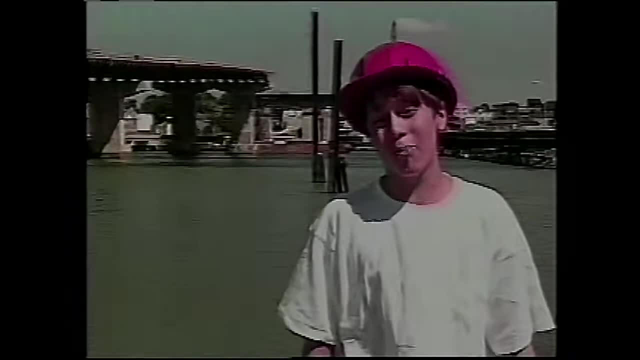 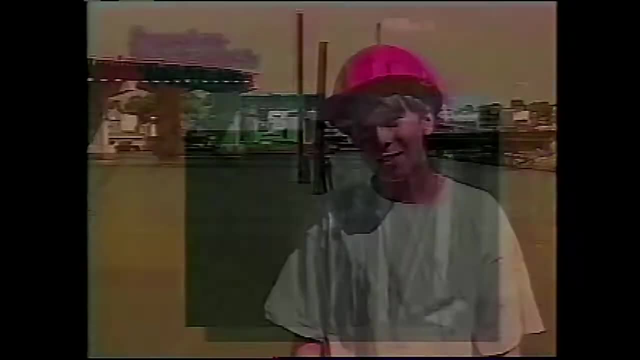 We had a real live construction. Workmen are building a beam bridge, called a fixed-span bridge. The bridge is being built so the road can cross over the water below Now. the first thing the workmen had to do was build the piers for the beams to span across. 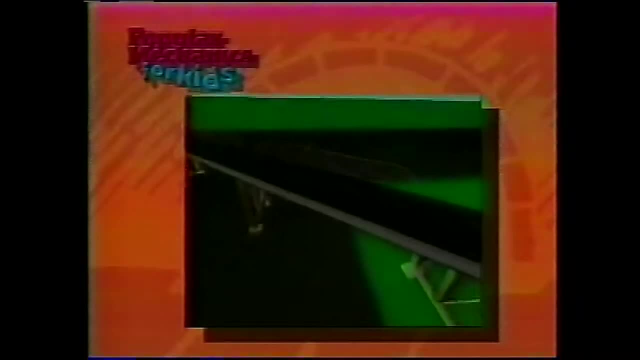 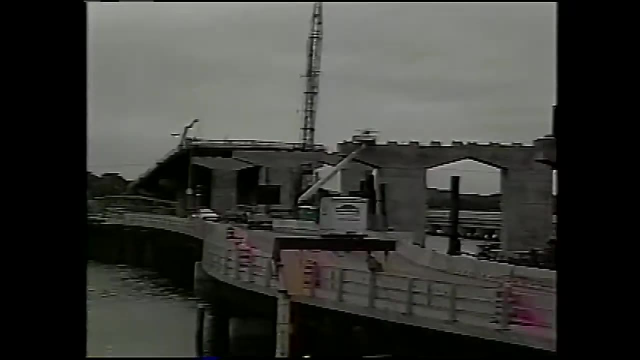 Now they are building one of the sections of bridge deck. Let's take a look. Yep, you're absolutely right, Mike. Little by little, they build the road across from one pier to the next For space shuttle fans. How Do They Build Spaceships? 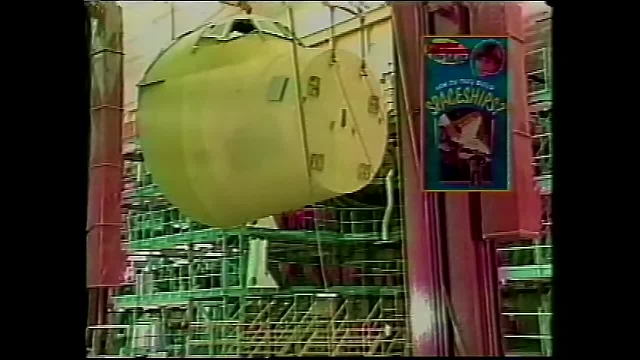 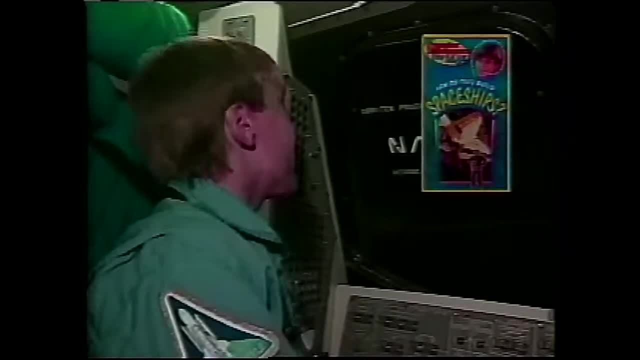 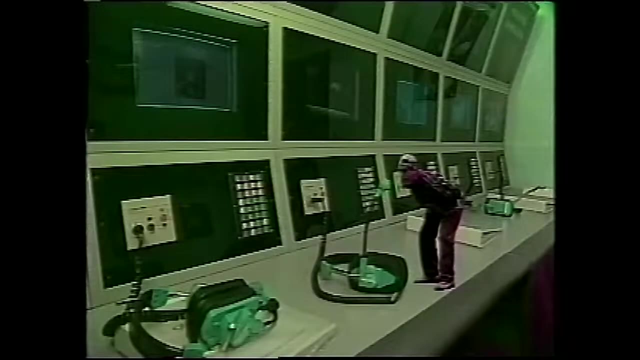 will take you on the ride of your life. Learn what's involved in building the space shuttle and what it takes to fly it. Hey, what's going on here? Hey, Pop, get me out of here. Mike, hang on, And don't forget to fasten your safety belt. 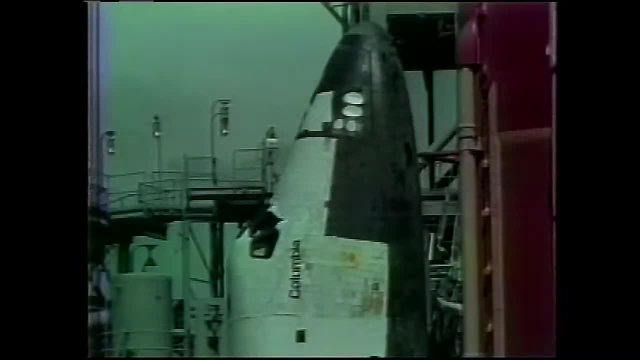 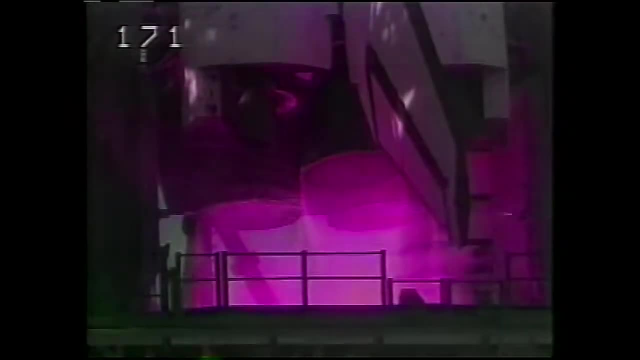 Pop, this isn't funny, Pop, I don't know how to fly this thing. T-minus ten, nine, eight, seven, six. Main engine start: Push the red button. Three engines up and burning The red button. Mike. 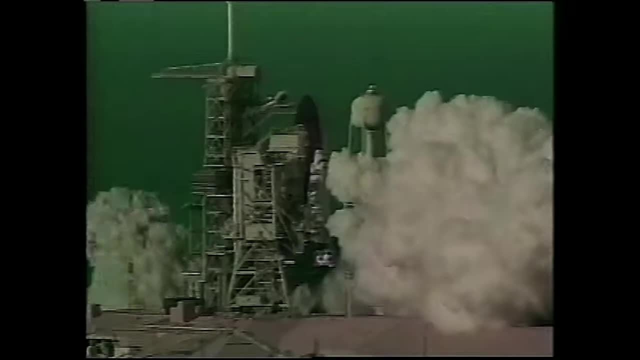 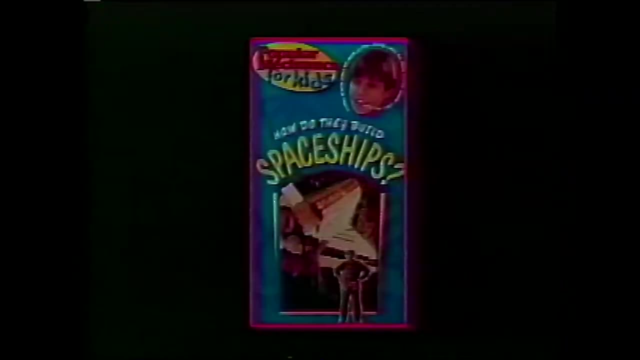 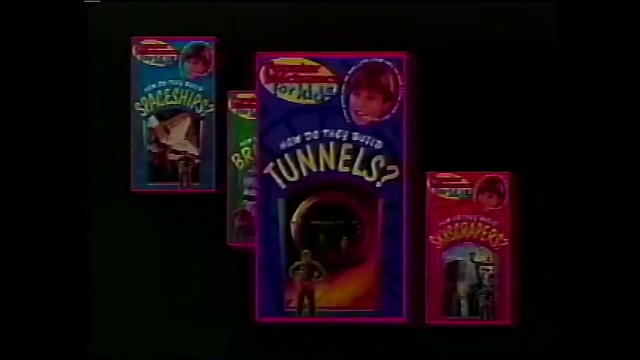 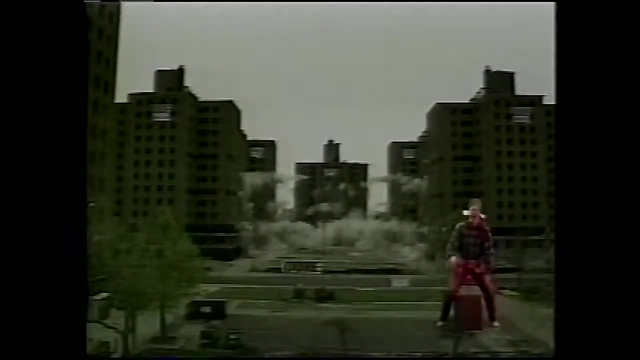 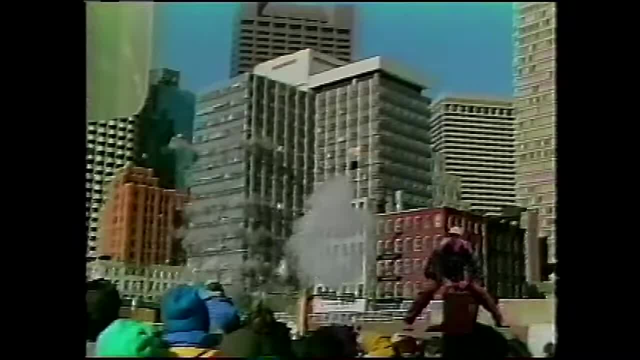 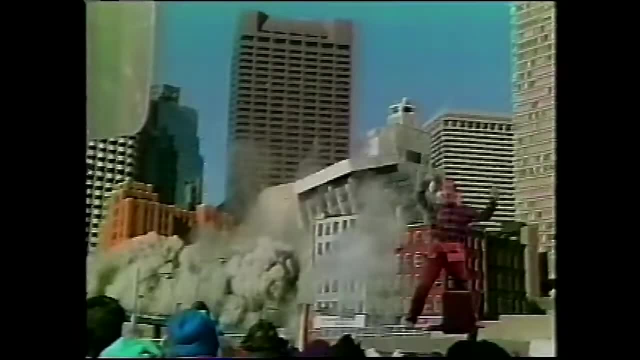 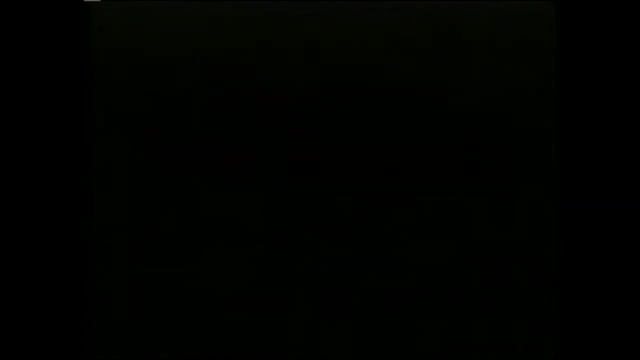 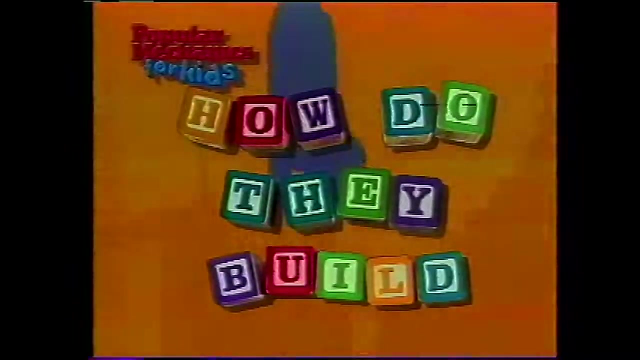 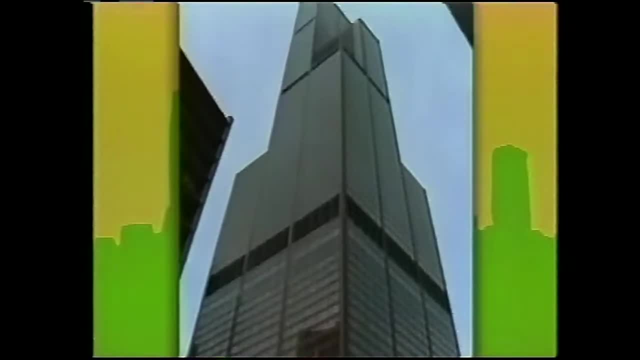 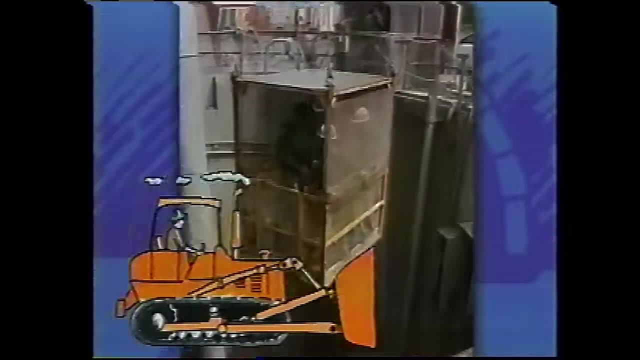 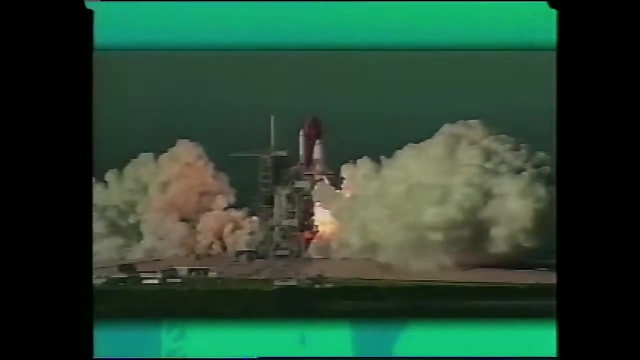 How do they tunnel below Where the water should flow, When it reaches so wide To the opposite side And when they rocket to space? I wonder how the food tastes. Czyli 환경을accept는 Spatial air designed By Alex Chiburu Ltd. I just want to know. 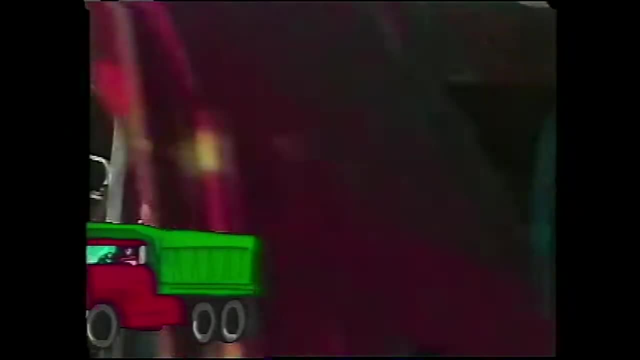 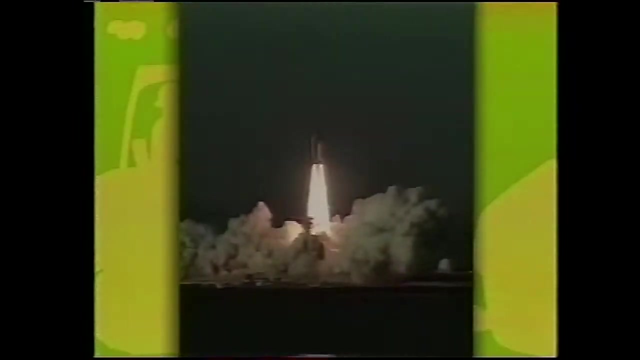 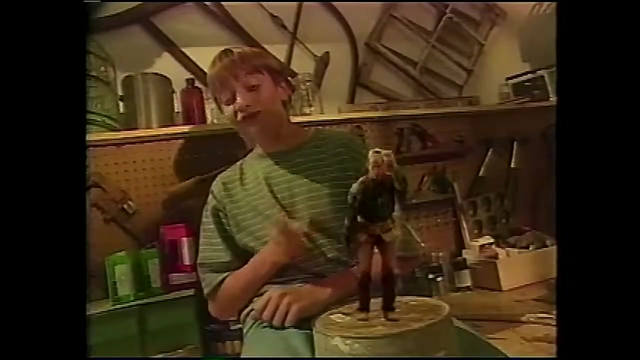 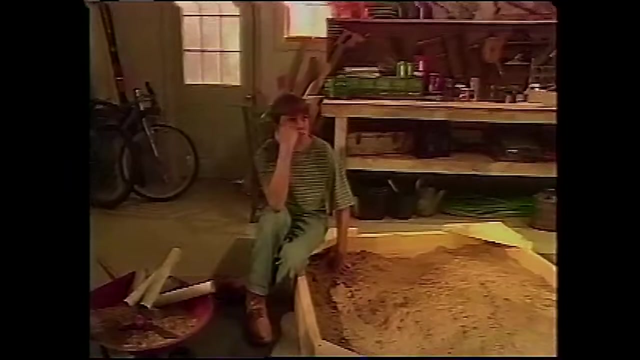 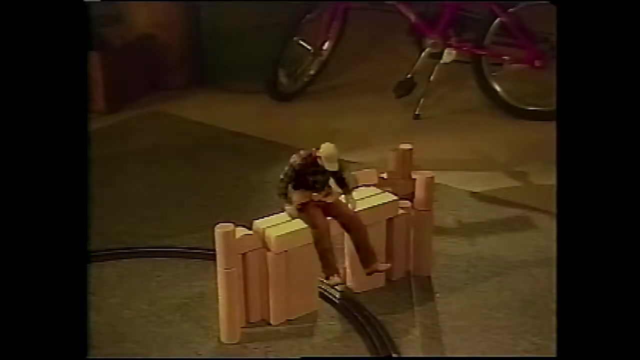 How do they build that, build that building so high? How do they build that bridge so wide? How do they build that, build that tunnel below And launch a space shuttle in the sky, In the sky. When all these questions come over me, Poppy tries to tell me why. 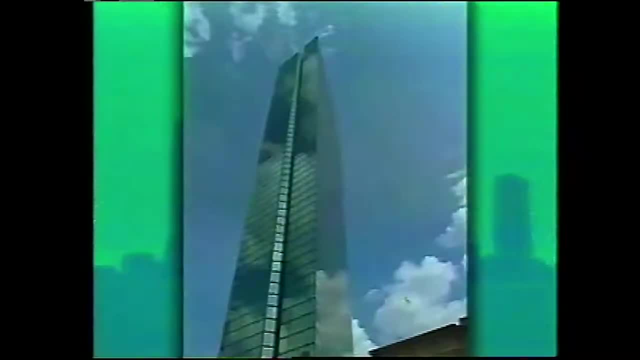 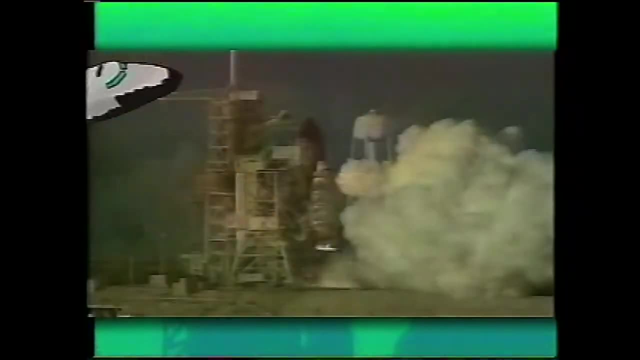 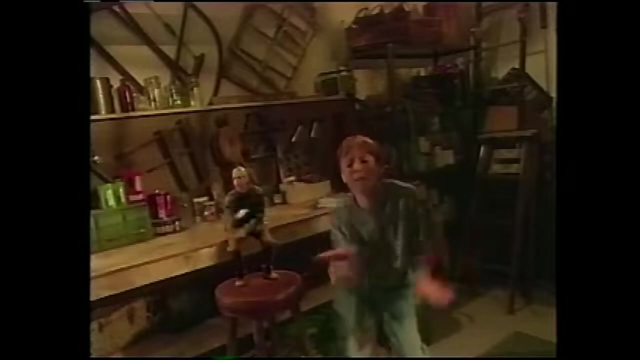 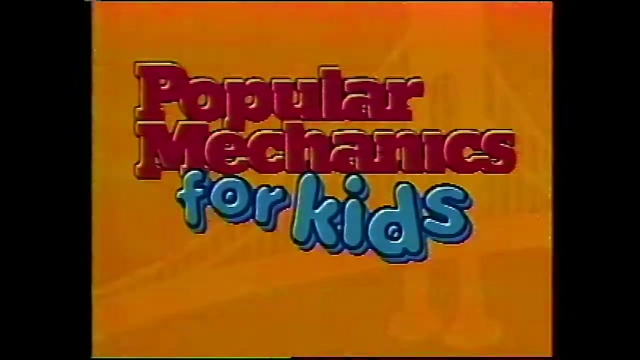 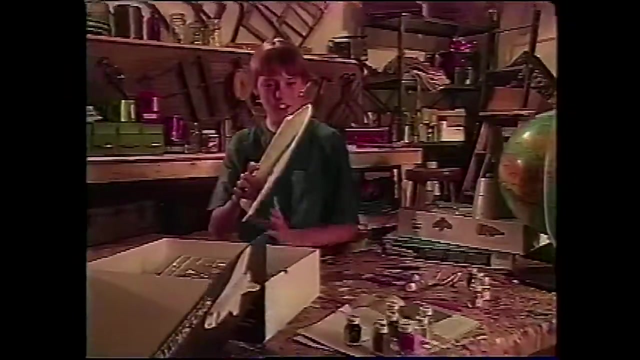 How do they build that? build that building so high? How do they build that bridge so wide? How do they build that? build that tunnel below And launch a space shuttle in the sky? How do they build that? This will be my best model yet, If I can just figure out how to put it together. 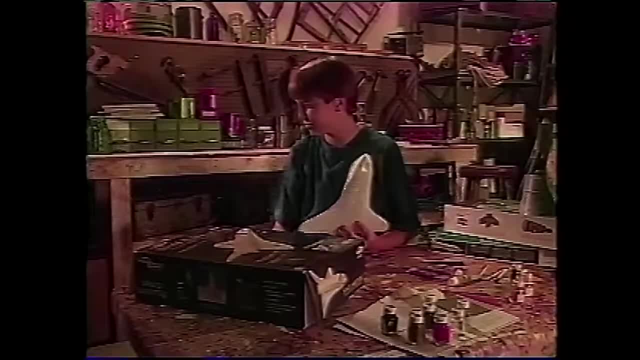 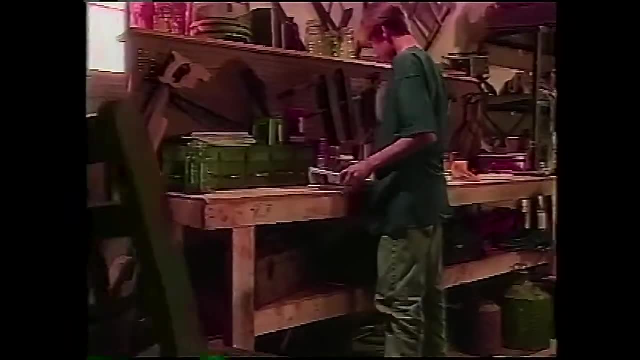 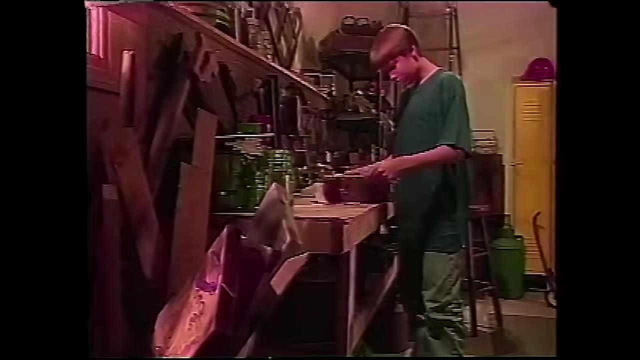 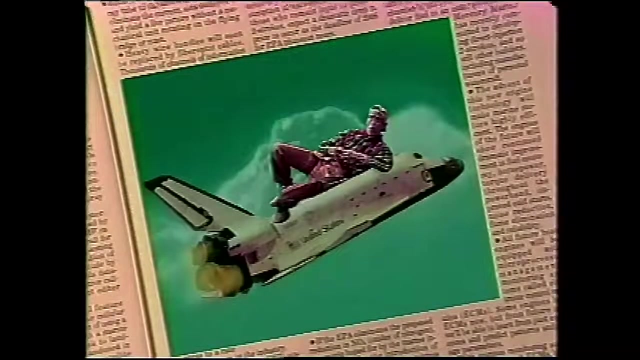 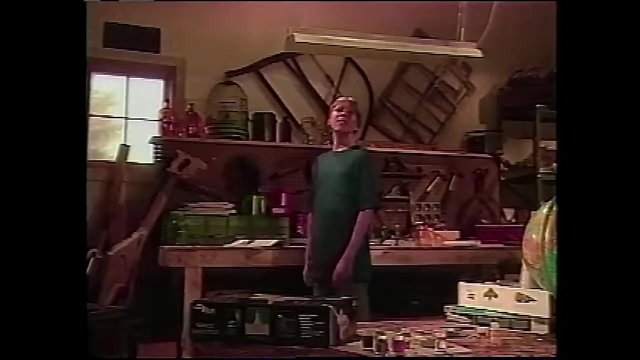 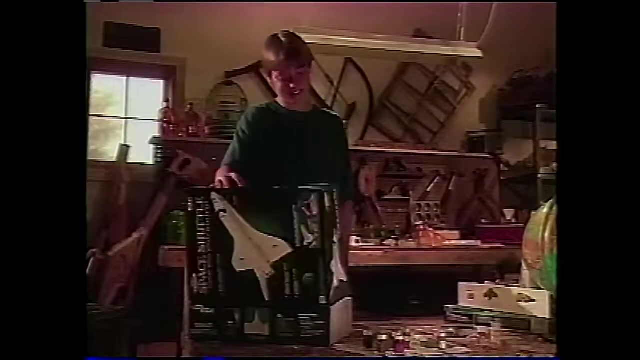 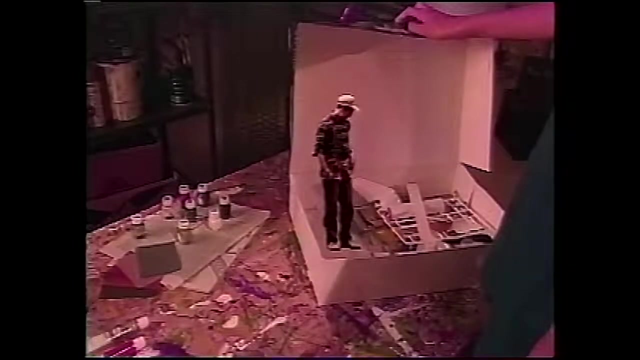 I have an idea. Pop, there you are. What are you doing? Don't you know? there's no air and space. Pop, Let me out of this thing. There you are Messed up on my landing coordinates. Hey, nice model. Yeah, but I can't figure out how to put it together. 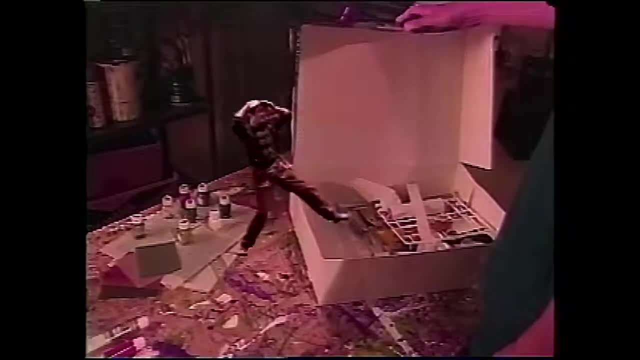 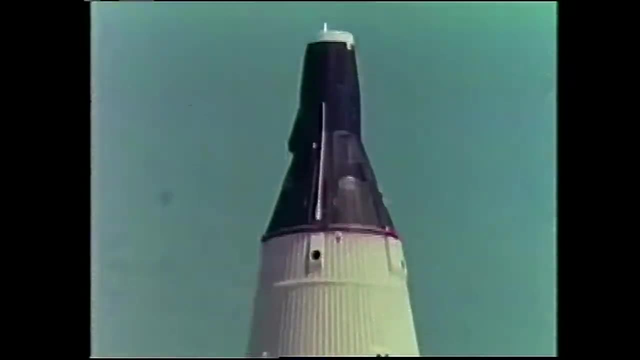 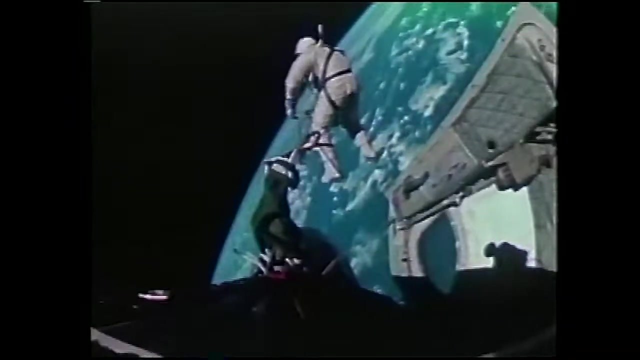 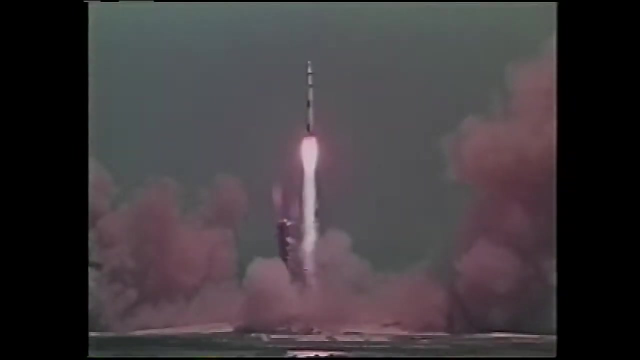 Well, I think I can help you. What you think? No, you are not. You're just a set of The Space Shuttle what astronauts use now to fly into space. Before the Space Shuttle, there were lots of different kinds of rockets and spaceships. 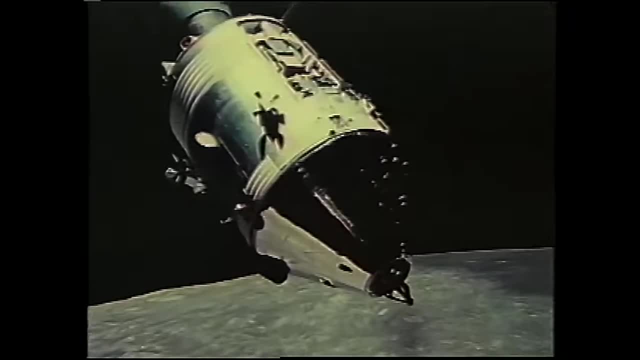 Who are those guys? They are some of the very first American astronauts. Astronauts had to learn a lot about what it was like in space, And each mission taught them a little bit more. The spaceships that the astronauts used changed as each mission got bigger and bigger. 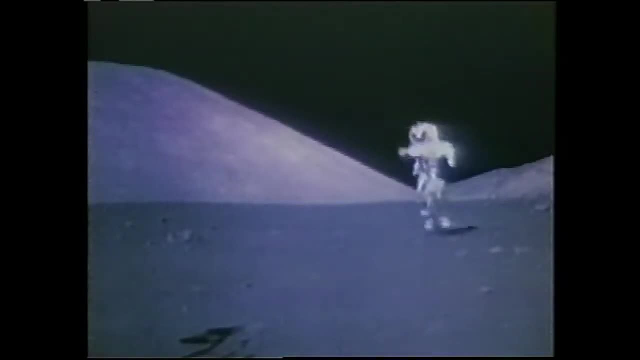 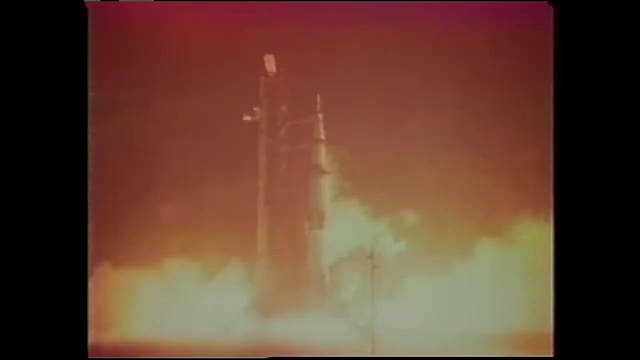 Boy. was that exciting, Cool. I'd love to drive a buggy on the moon. So would a lot of people. These days, lots of astronauts go up in the space shuttle Now. they're very lucky and they're very important scientists. 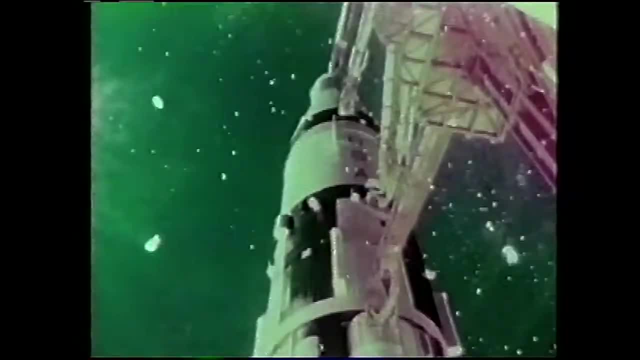 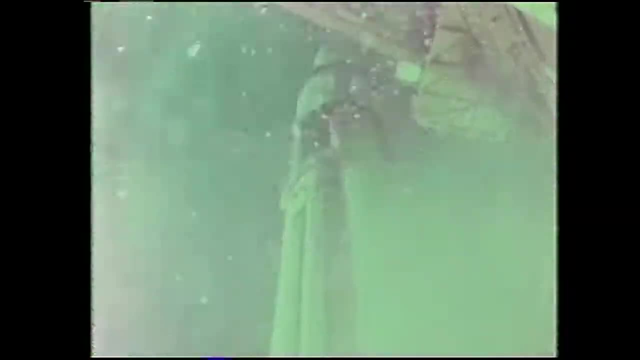 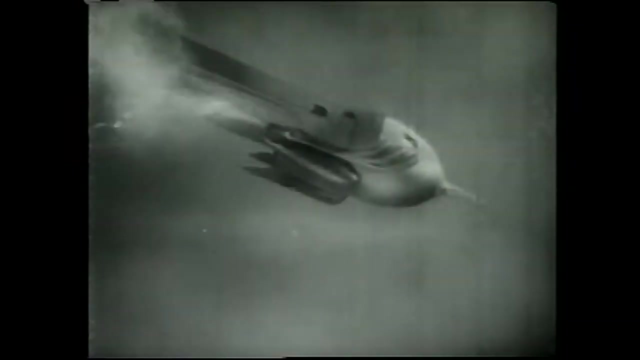 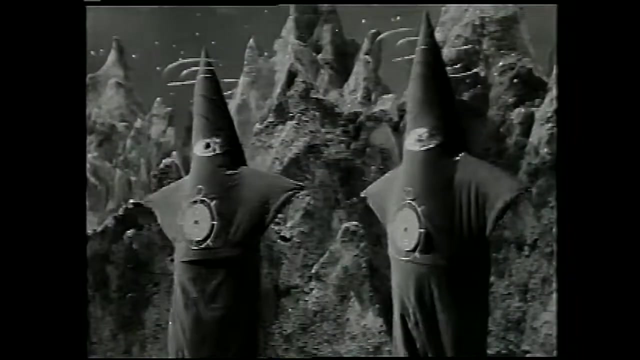 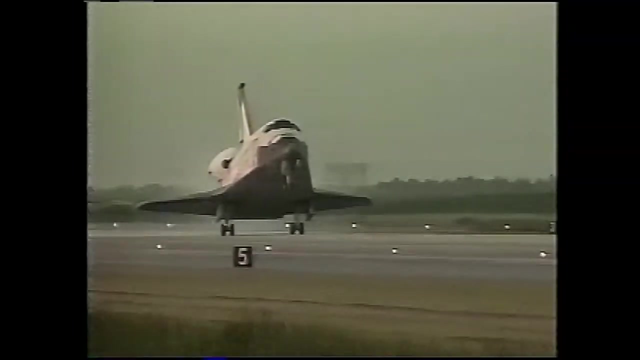 But those early astronauts were real heroes because nobody had ever done what they were doing before. Hey, that's not a real spaceship. No, it's pretty funny to see how we imagine spaceships and space people to look. huh, Yeah, Hey, the space shuttle's landing. 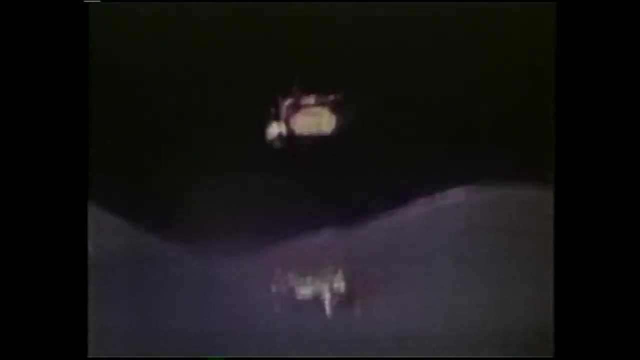 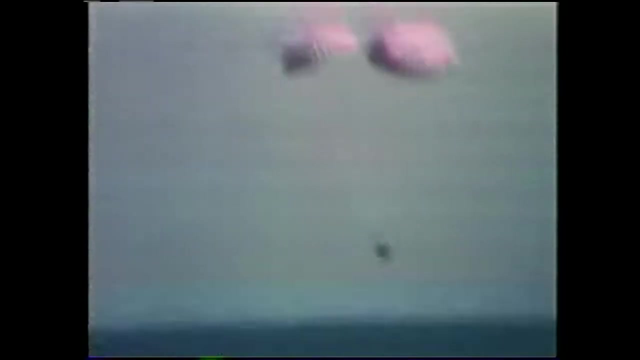 But wait, what's that? That's the lunar lander blasting off from the moon. We'll learn more about that later. Did you know that the space shuttle is the first spaceship that lands back on Earth and can be used again? All the earlier spaceships splashed down in the ocean. 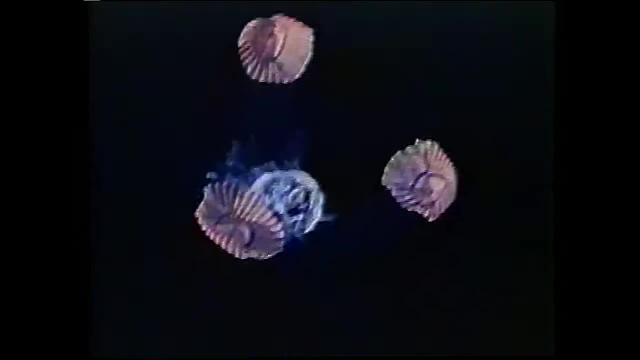 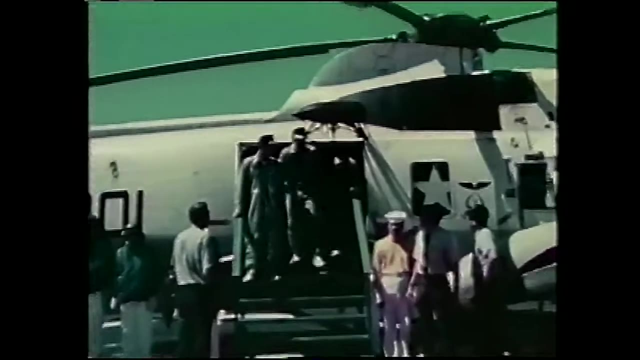 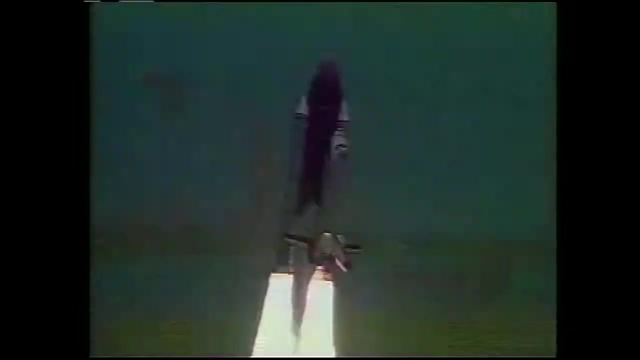 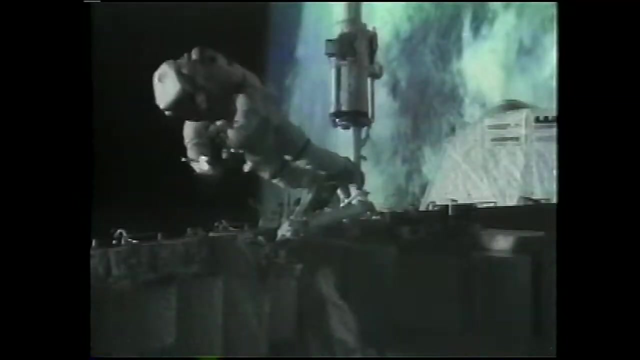 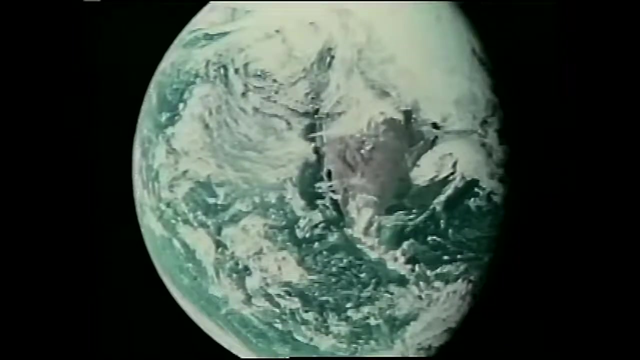 and were never used again. How'd they get the astronauts out? Big Coast Guard helicopters picked them up. See, There goes the shuttle. Yep, there it goes. Pretty nice view from up here, though. huh Yeah, So you were thinking it was hard to build your model. 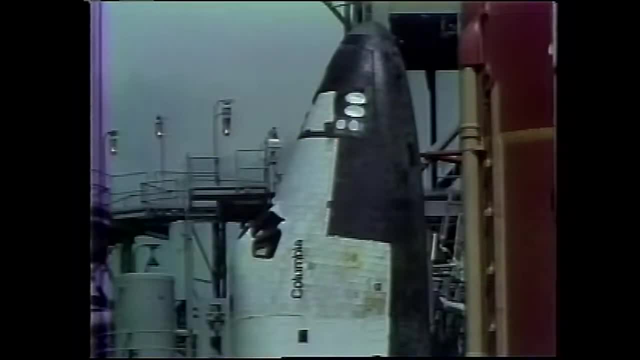 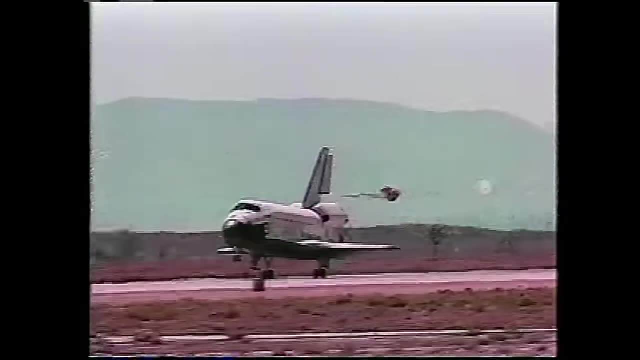 Imagine what it takes to build a real space shuttle. Wow, how'd they do it? Building that machine is one of the most amazing achievements in human history. It took years and years of research, testing and designing, But once they figured it all out, 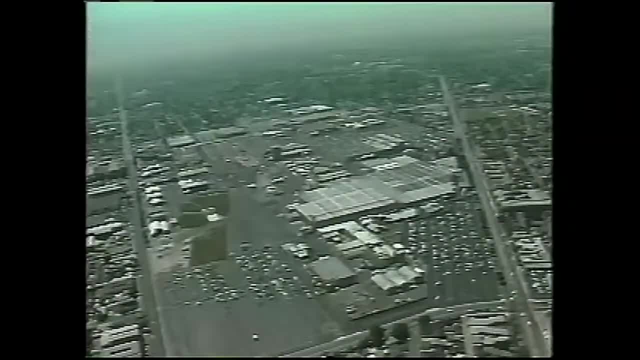 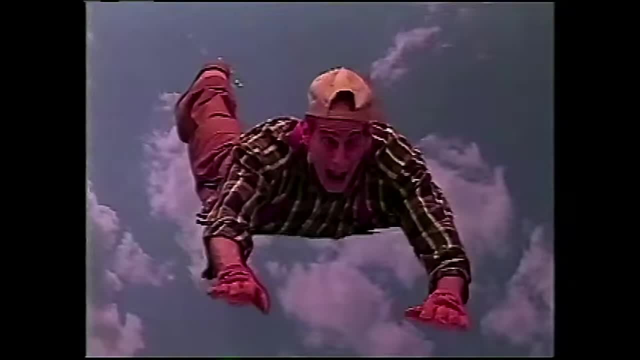 it was just like building a really, really complicated model. You're kidding? No, it's true. Here Over Rockwell International, the place where they build them, so I could check it all out. See, Here they are assembling the big pieces of the space shuttle. 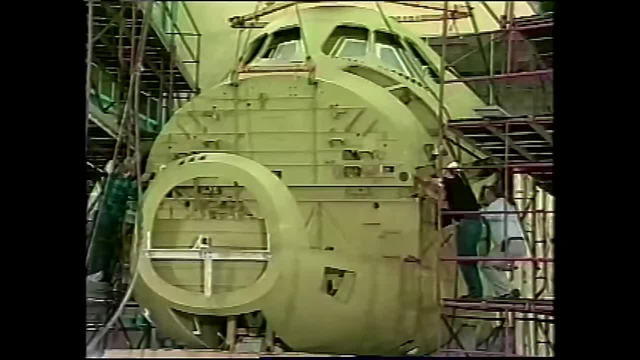 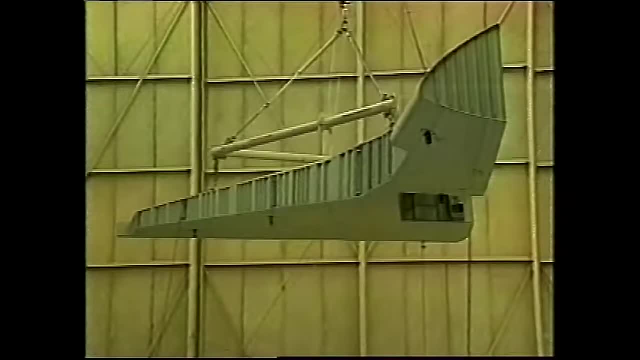 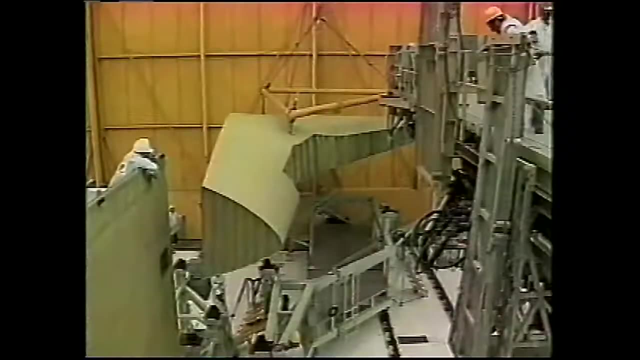 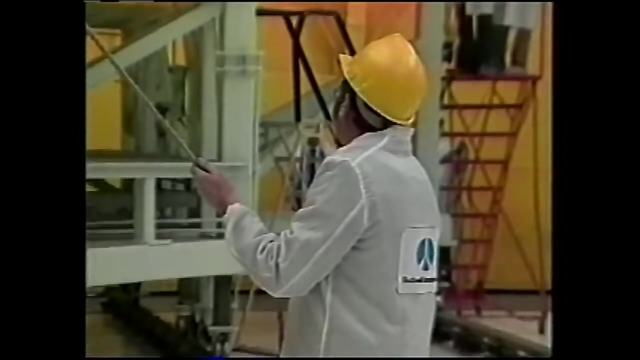 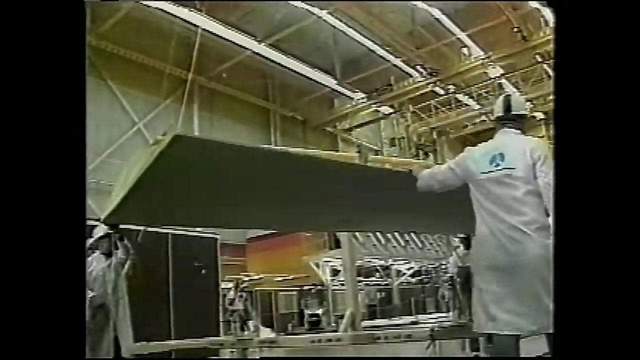 Right now they're putting the cockpit on. Here comes one of the wings, And now they are securing it in place. Oops, There's the other wing. There's one of the wing flaps that helps the astronauts steer. Looks like they're missing a window. 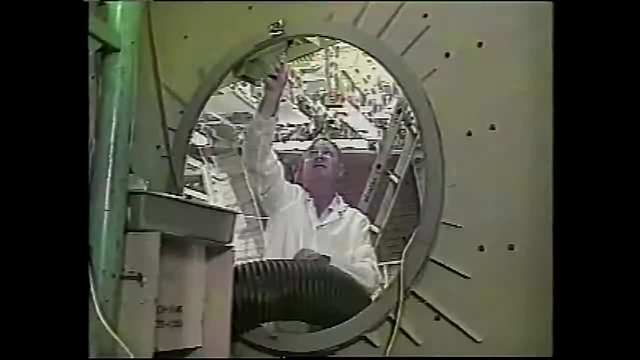 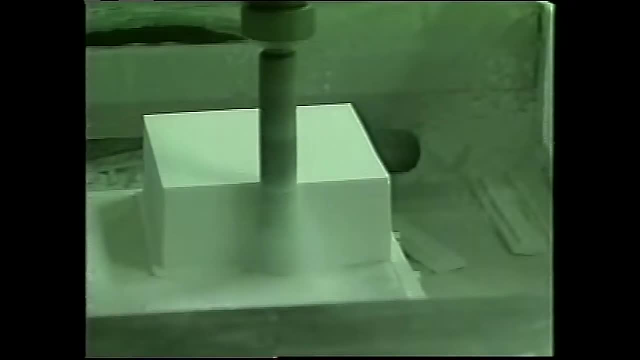 Yep, Piece by piece, they put it together. What's that? That's a tile. When the space shuttle re-enters the Earth's atmosphere, it gets really hot. So they cover the entire bottom of the shuttle with these special tiles. 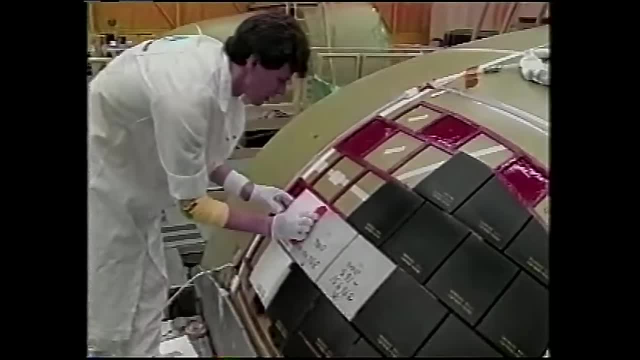 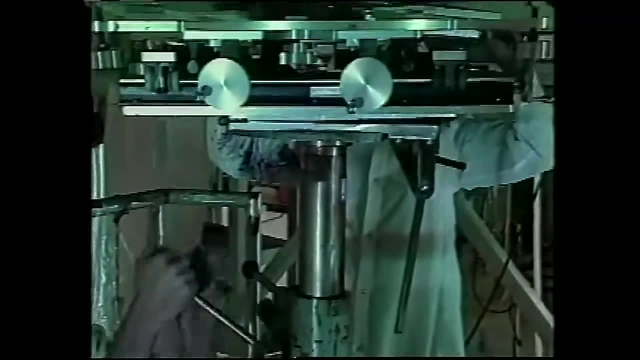 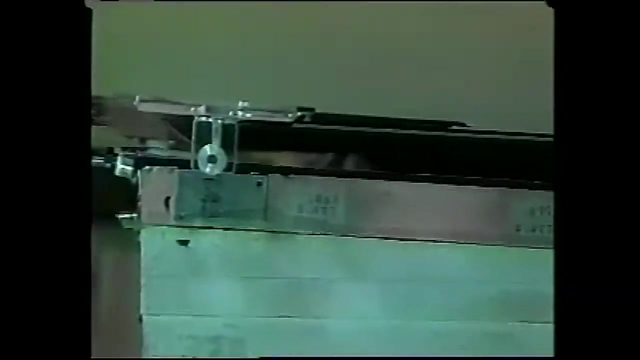 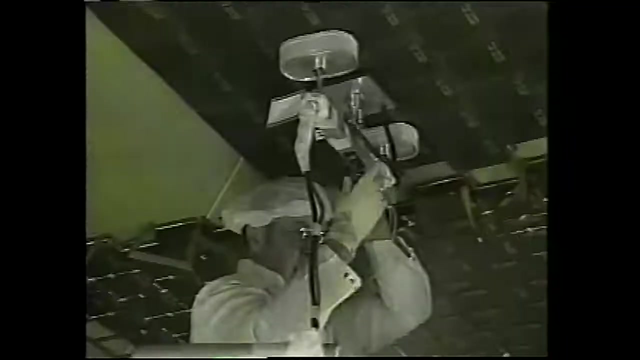 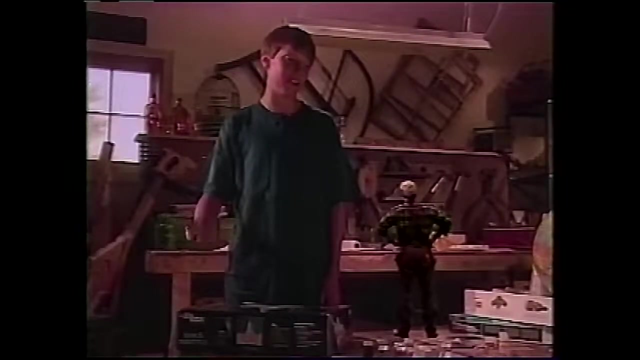 that protect the shuttle from the heat? Are all those tiles? Yep, And they have to be very careful putting them on. so they use these specially designed machines, And I thought I had problems. I think I'll just read the directions and build my little model. 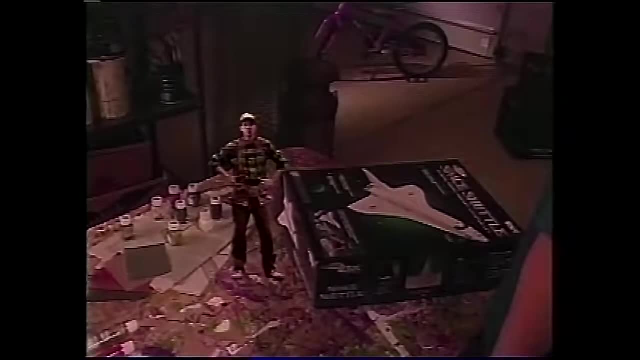 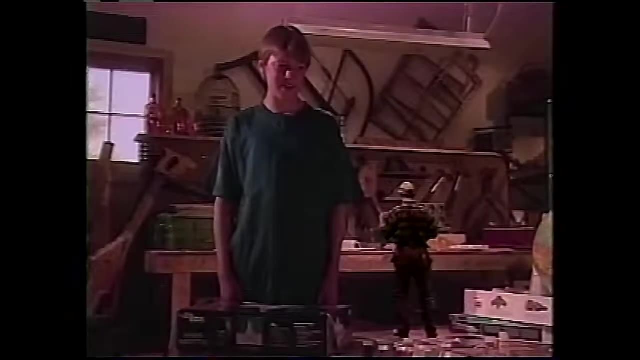 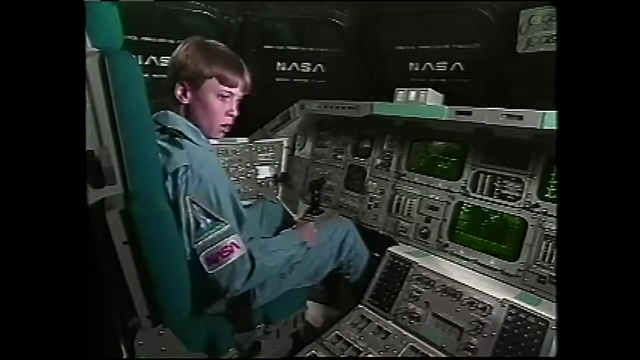 Why are the real ones so complicated? You'd understand if you ever took a ride in one. Hey, why not, Pop? what are you doing? Hey, hey, what's going on here? Hey, Pop, get me out of here. 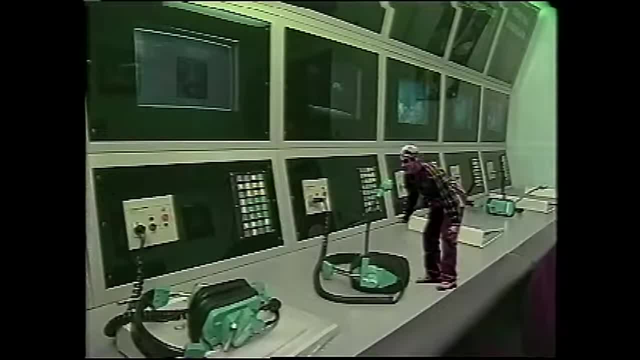 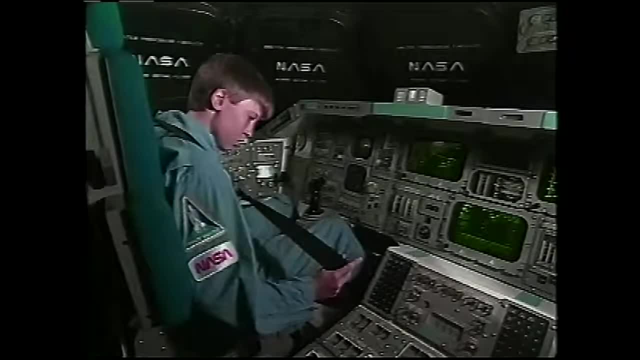 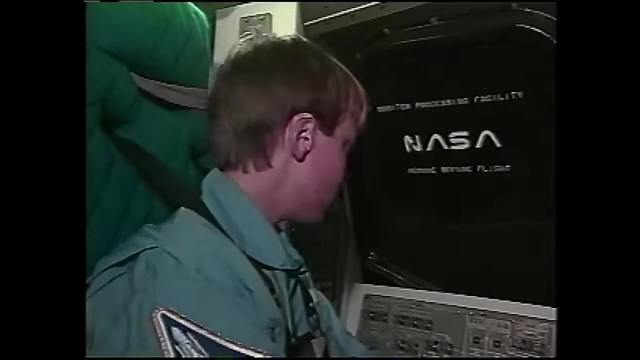 Mike, hang on And don't forget to fasten your safety belt. Pop, this isn't funny, Pop, I don't know how to fly this thing. D minus ten, nine, eight, seven, six. Don't forget, push the red button. 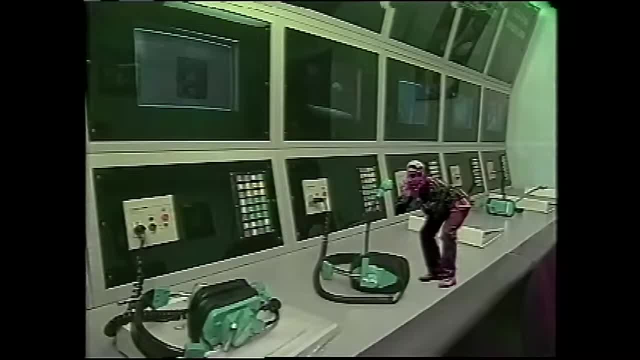 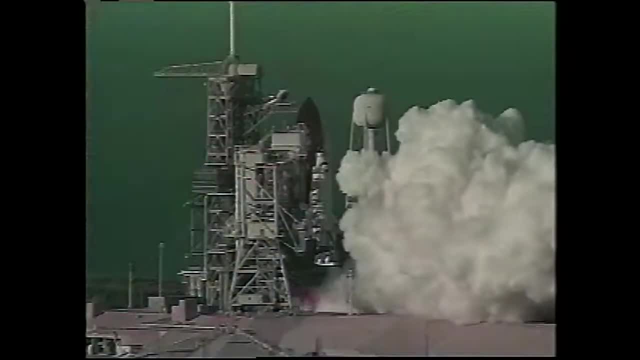 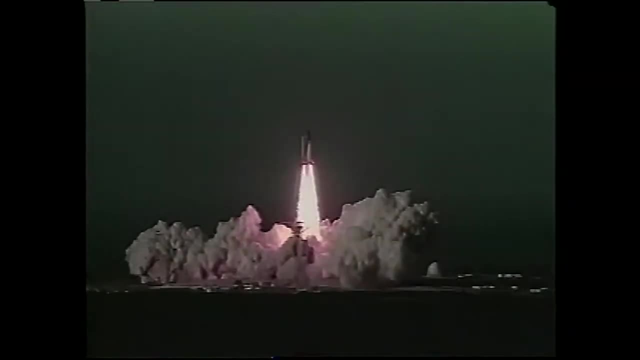 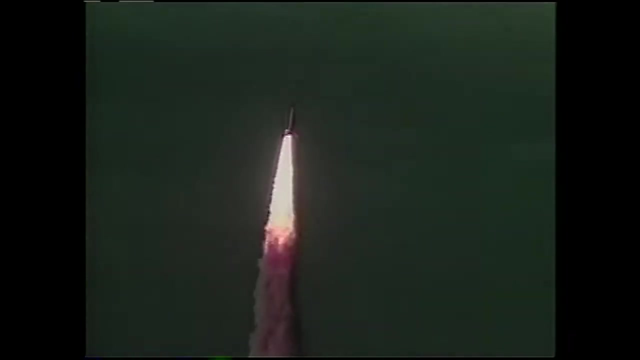 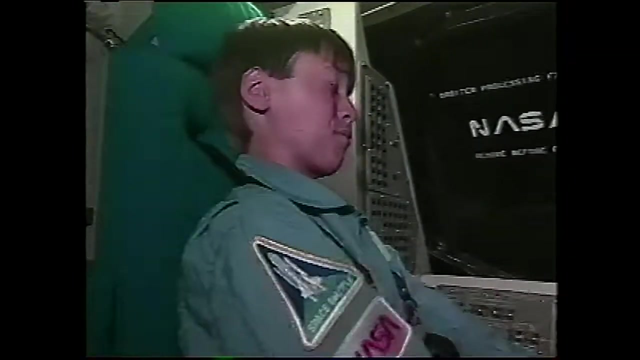 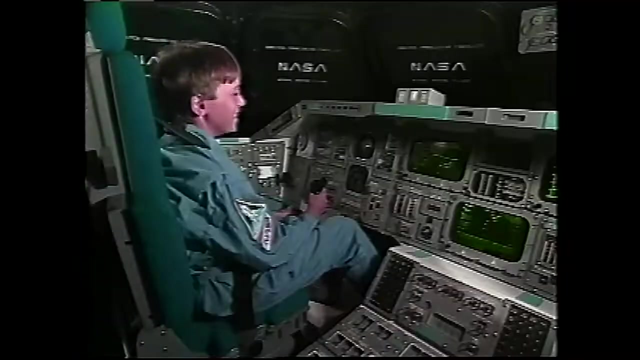 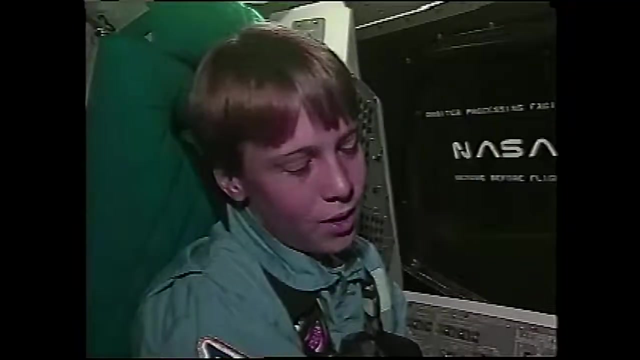 Three engines up and burning The red button. Mike Where Pop where Three? two, one Liftoff of Space Shuttle Discovery. 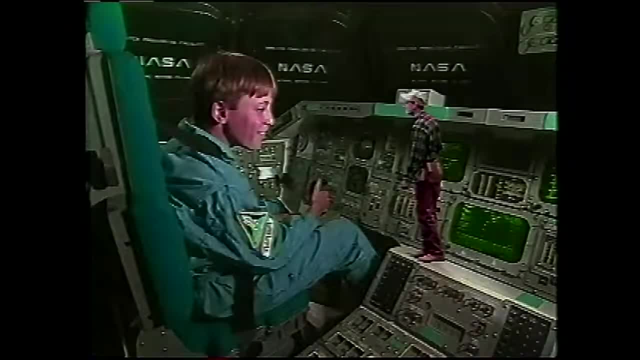 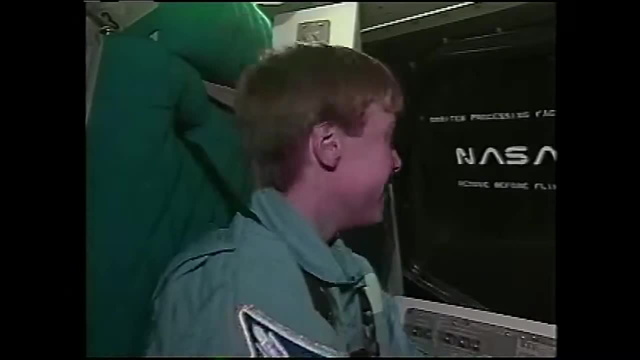 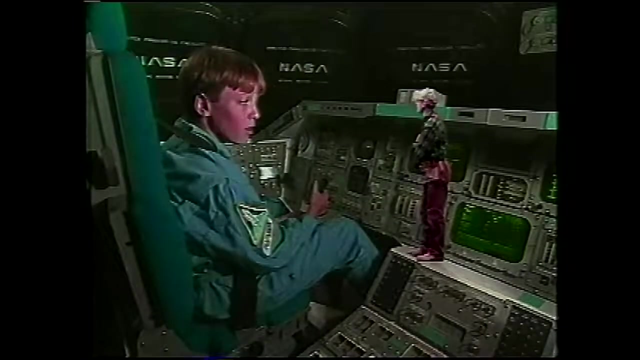 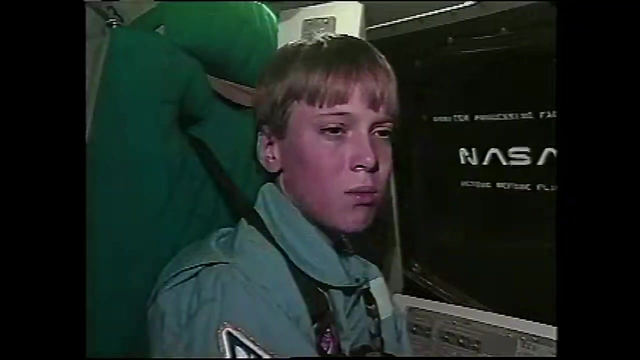 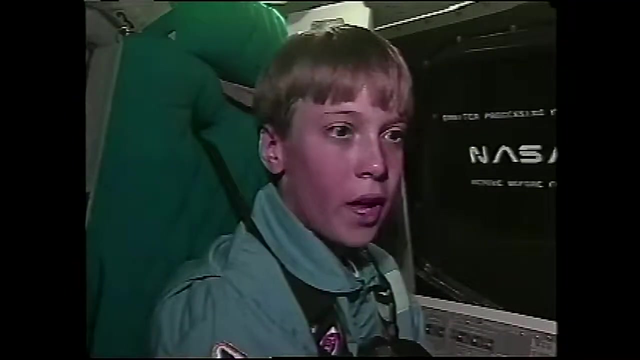 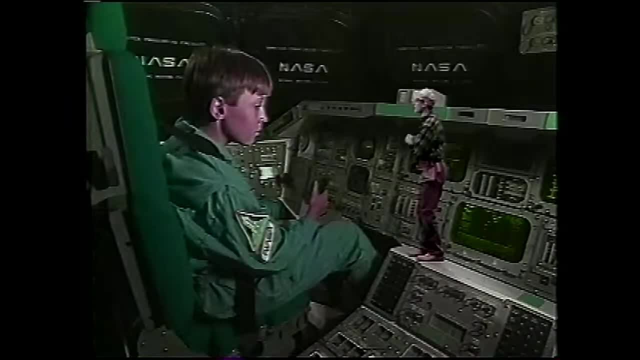 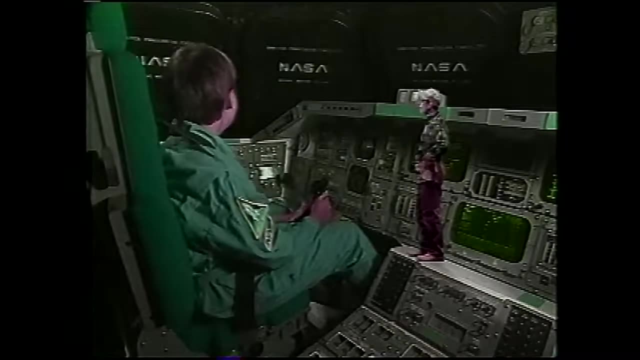 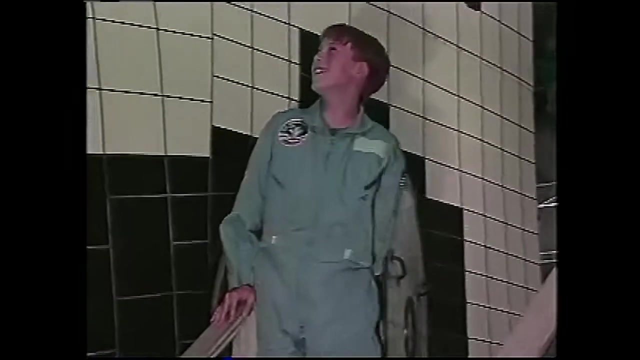 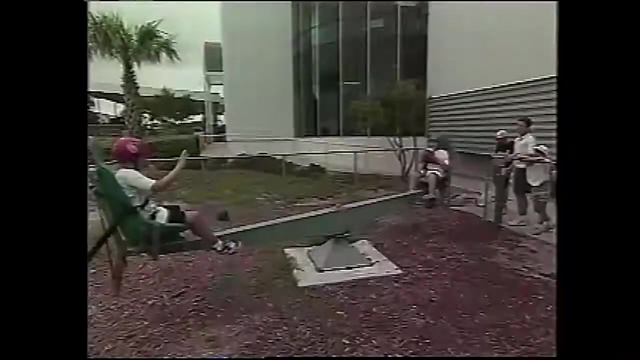 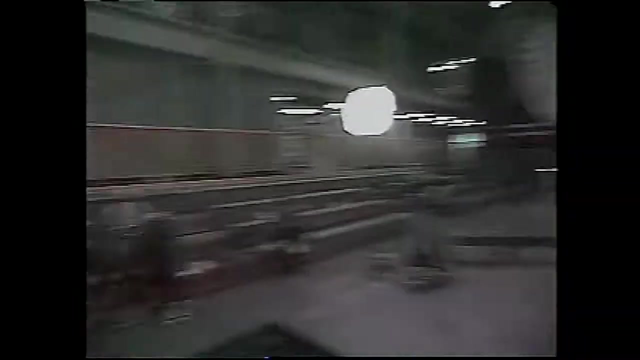 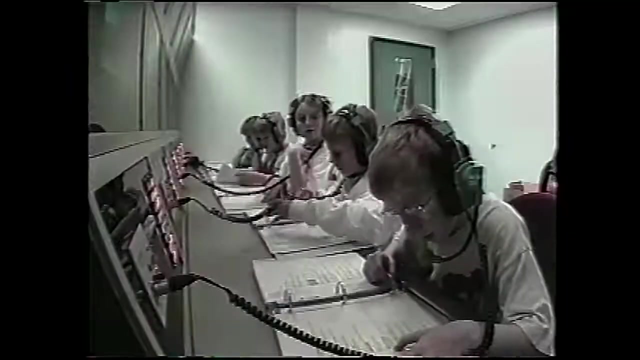 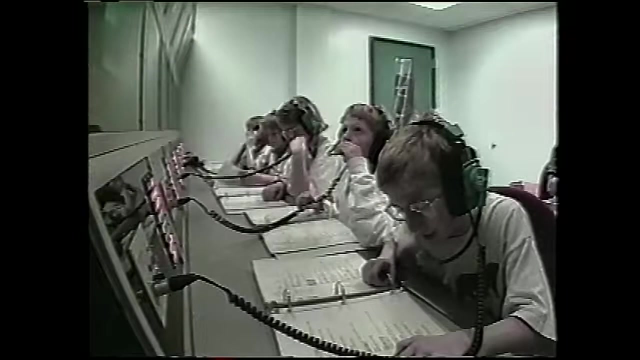 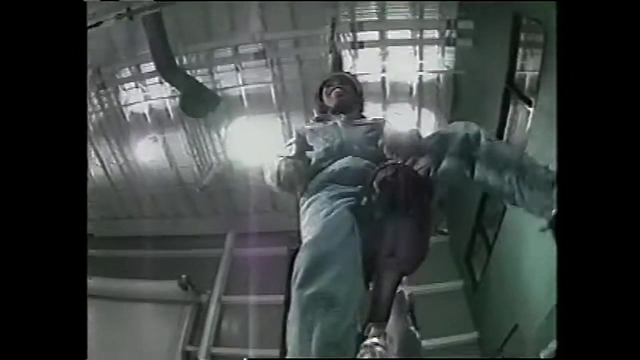 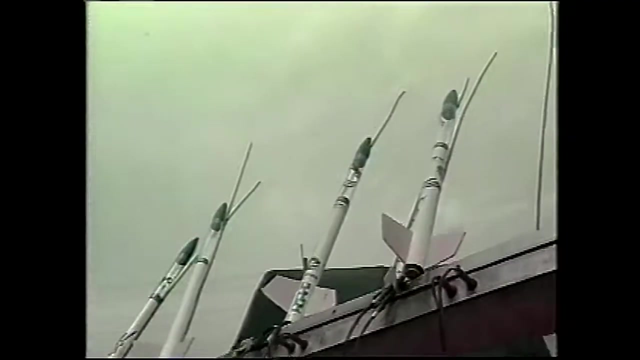 T-minus 10 seconds: 7, 7, engine start. 3, 2, booster ignition liftoff. Automatic separation in 30 seconds: 5, 4, 3, 2, 1, ignition. 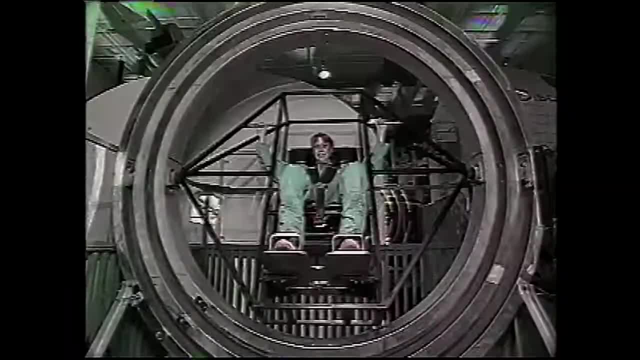 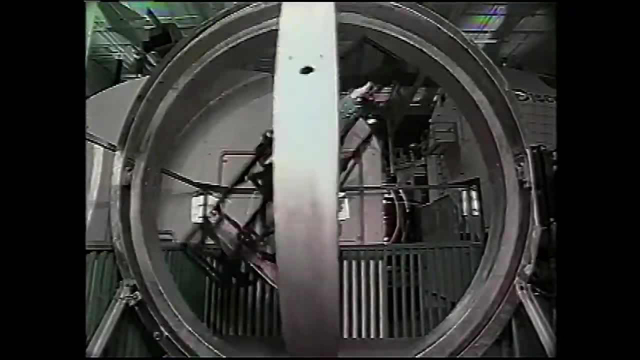 When astronauts need to learn what it's like to be in space, they use things called simulators. This one makes you feel like you're on a spaceship that's out of control. I was just trying to keep my stomach in control, so I didn't throw up. 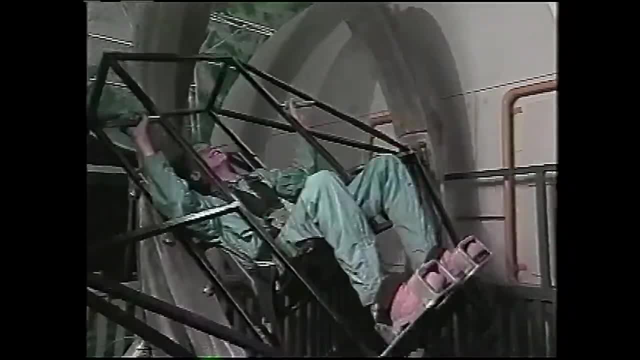 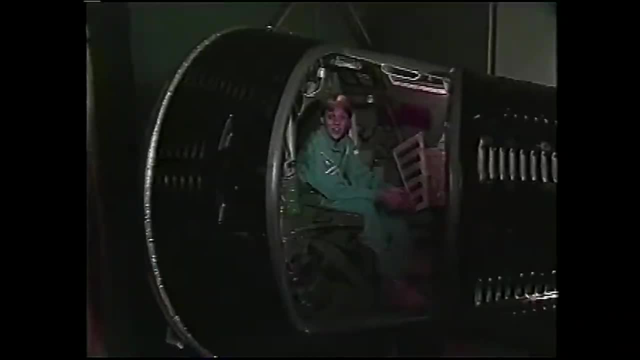 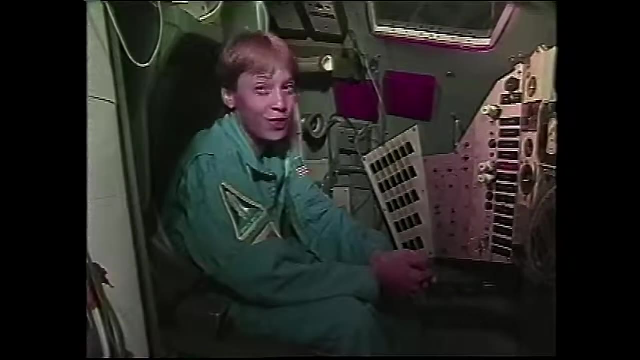 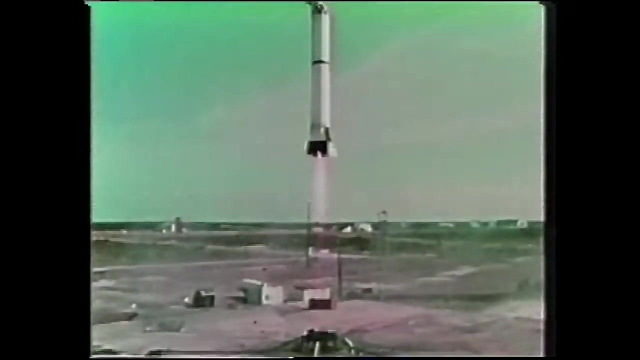 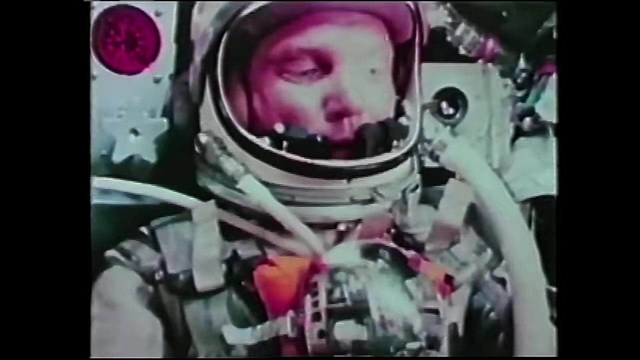 Man, was I glad when that one was over. This is a Mercury space capsule. Mercury was the first American space program. Only one man could fly into orbit in this tiny capsule. Mercury was America's first mission that took people up into space, and it lasted a whole five years, from 1958 to 1963.. 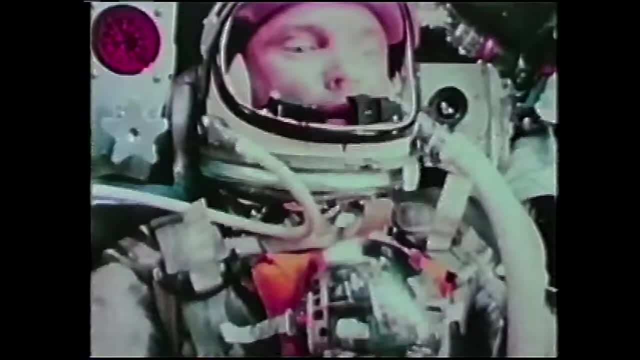 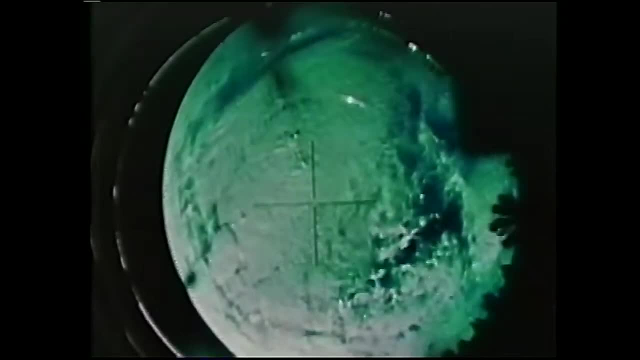 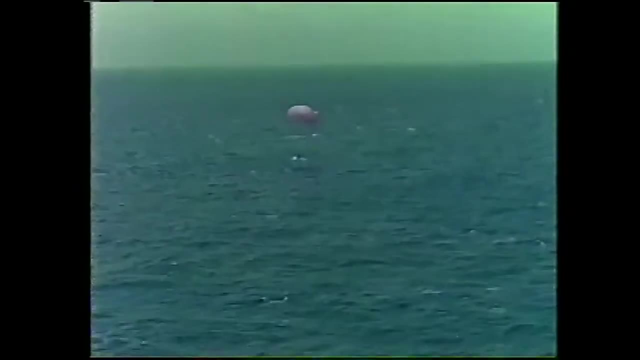 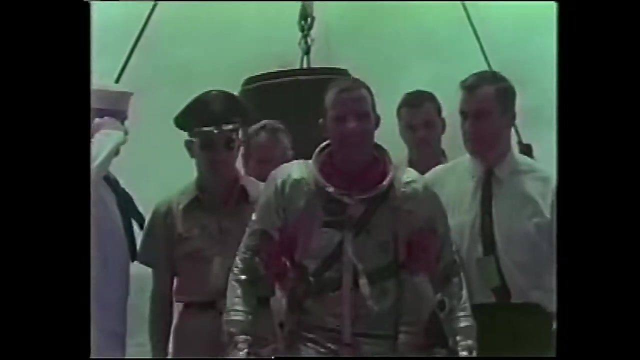 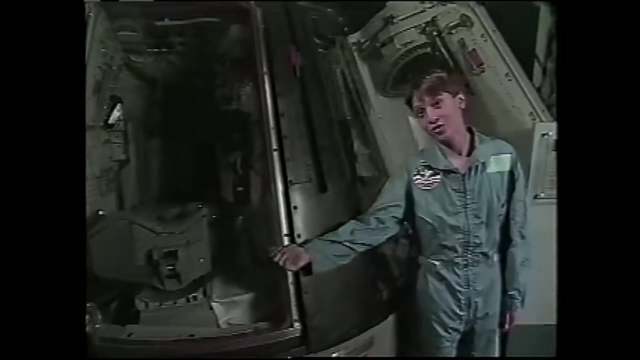 The Mercury program proved that people could rocket up into space, orbit the Earth and return safely. Oh, that view is tremendous. Roger Understand, go for at least seven orbits. Orbiting the Earth means going around and around. Next came Gemini, with a space capsule big enough for two astronauts. 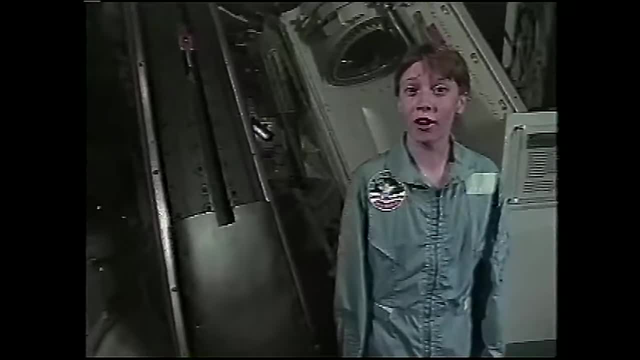 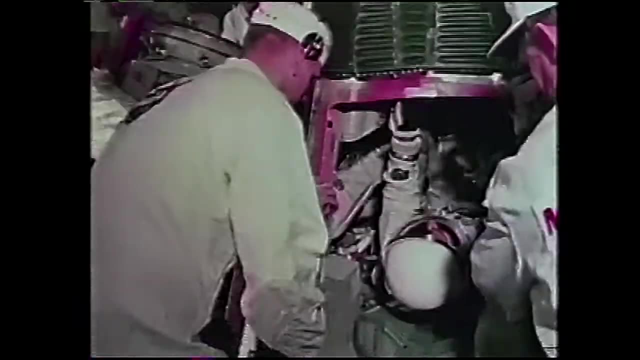 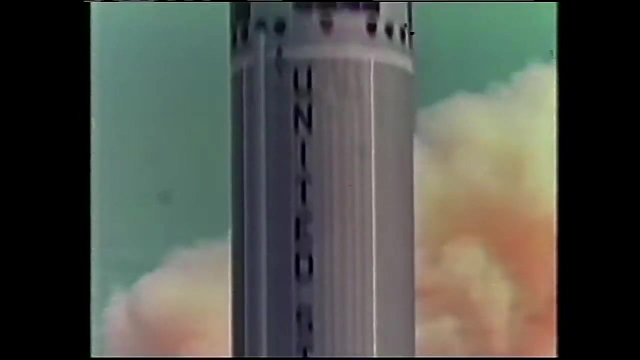 The Gemini program had a lot of firsts: The first American to walk in space and the first time two spacecrafts docked in space. Look at the astronauts squeezed into that capsule That's smaller than my closet. In the Gemini program they practiced a lot of the stuff. 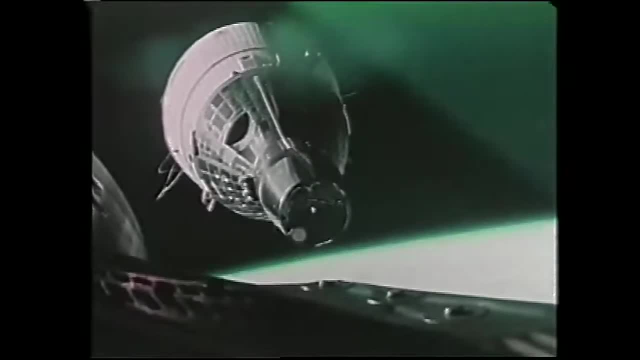 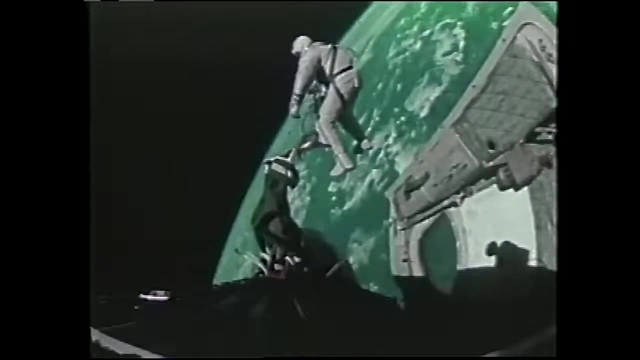 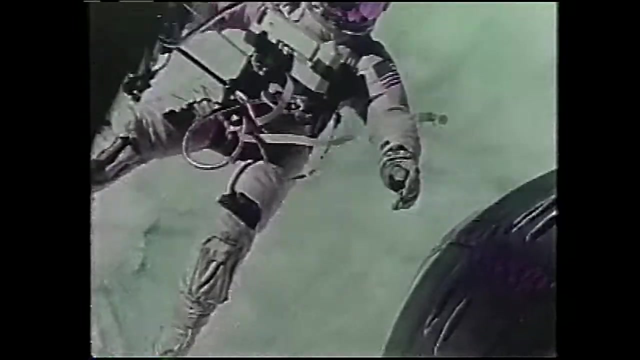 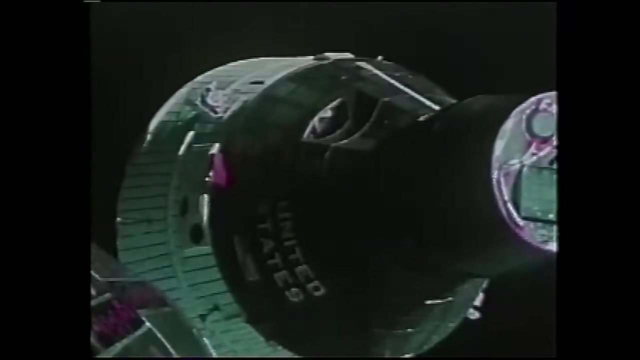 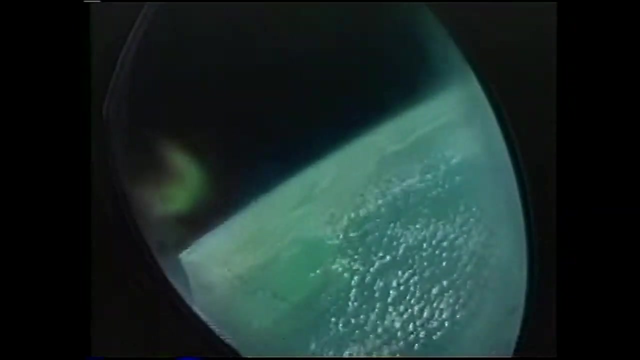 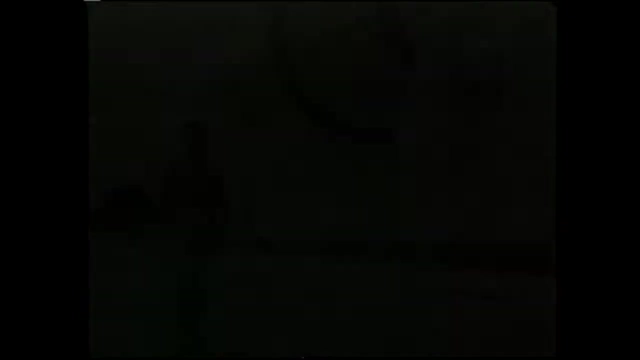 they were going to need to do in the Apollo moon missions. We can now very clearly see the horizon scanners operating: Roger Jim, Gemini 12,, Gemini 12.. The Apollo missions were even more ambitious. They were the missions that sent three men to space. 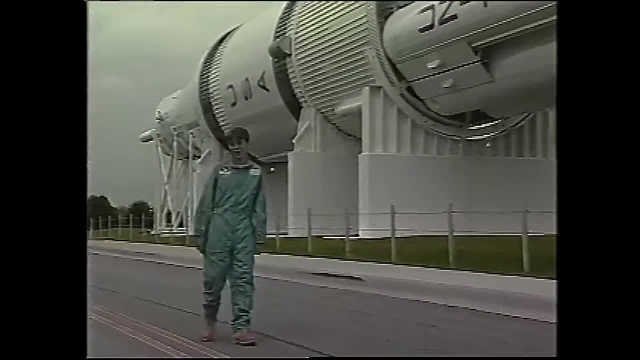 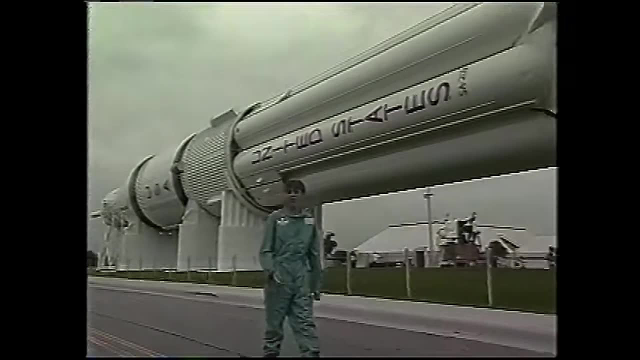 for the first time. They were the missions that sent three men to the moon and back again. They actually went in two spaceships: the space capsule and the lunar lander. One man stayed all alone in the capsule, while the other two went down to the moon's surface. 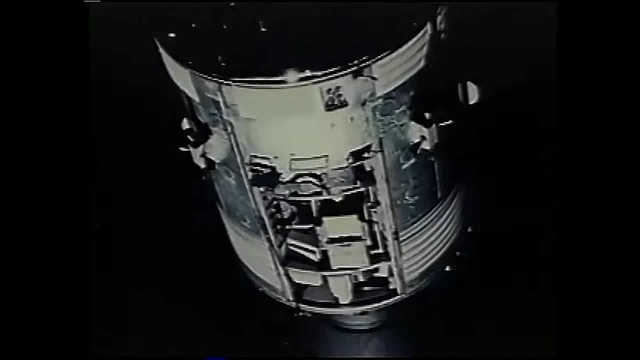 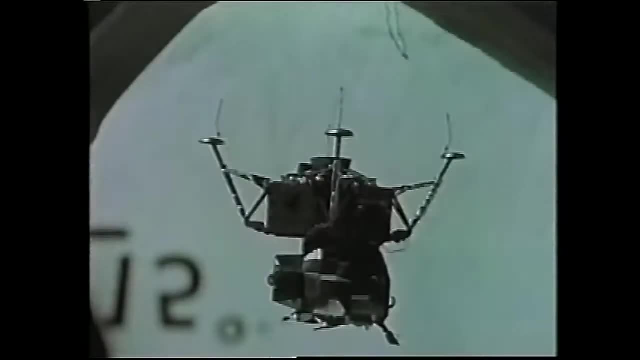 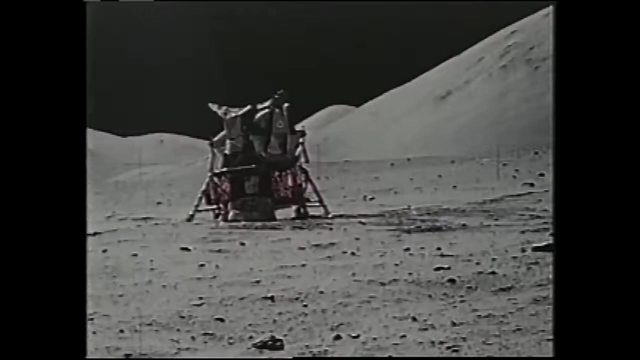 There's the capsule that orbited around the moon And there's the lunar lander, the funny-looking spaceship that actually landed on the moon. Neil Armstrong was probably the most famous astronaut. He was the first man to walk on the moon. Here's what he said when he stepped out of the lunar lander: 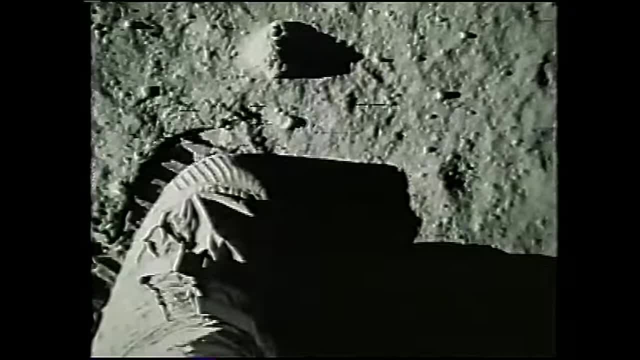 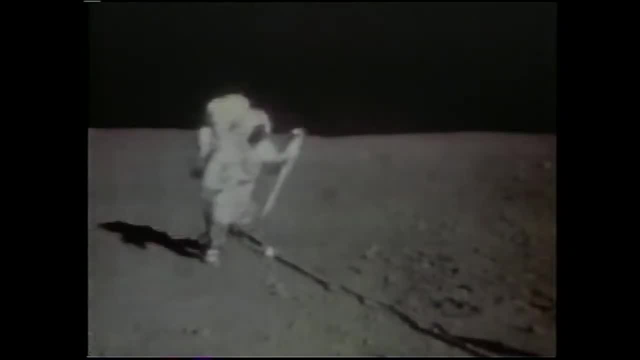 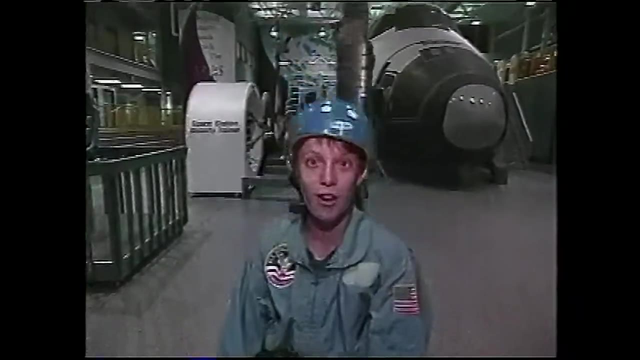 That's one small step for man, one giant leap for mankind. This is a 1-6 simulator. It teaches you how to walk on the moon, which has much less gravity. If you're looking for the most creative, creative trick. 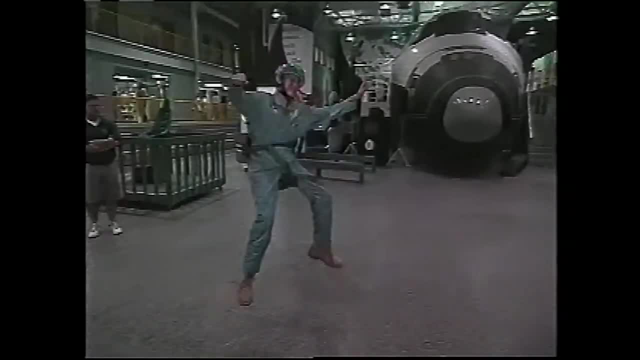 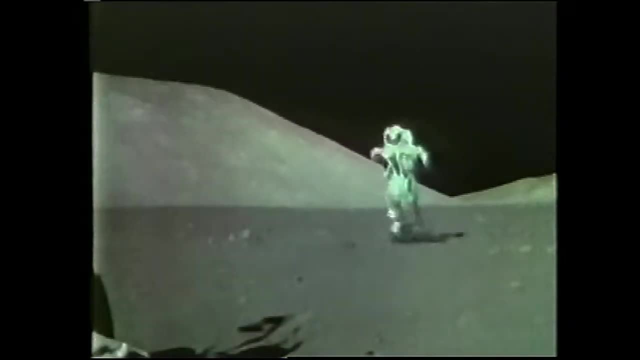 and she is: this, is it? We're doing one of those same tests we did when we were at NASA, When they're starting to come to us with NASA, we had to go down to the moon. It's a little confusing. Who knows? 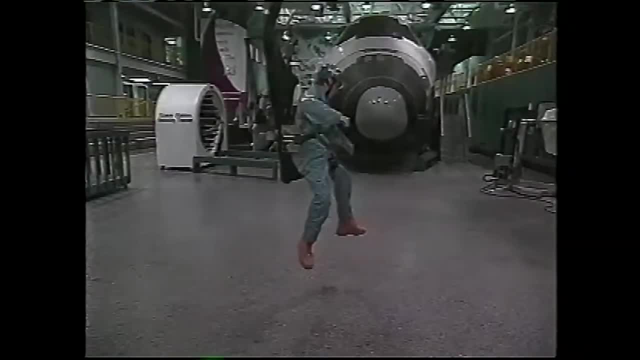 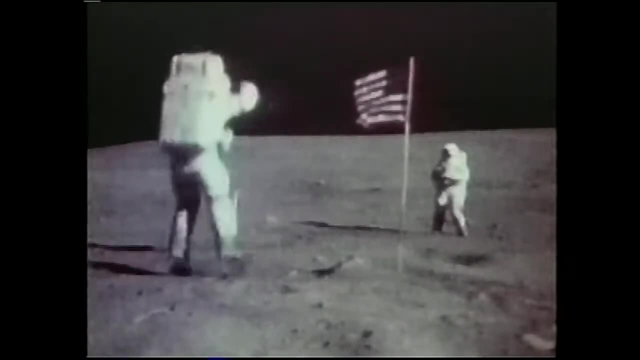 I mean, we can make mistakes, mistakes, mistakes. That's not happening. You can make mistakes, That's not happening. But if you do the same thing, you do the same thing When we're at NASA. we can make mistakes. 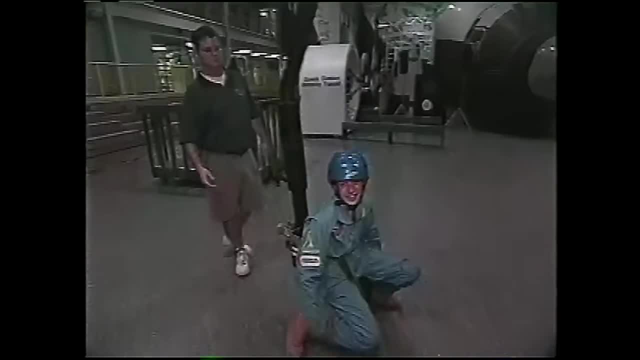 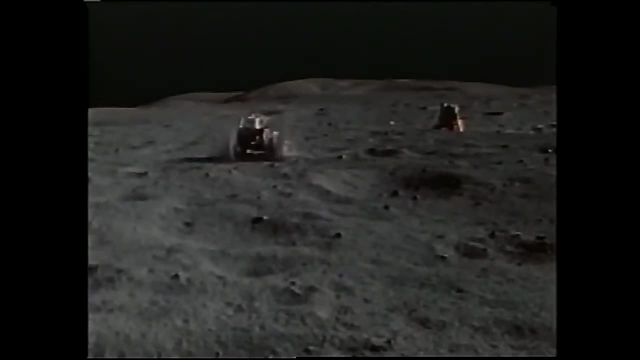 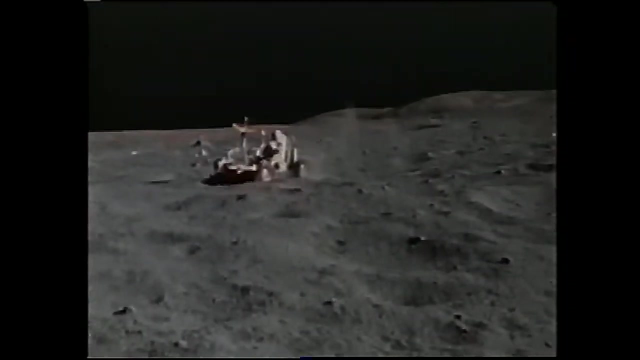 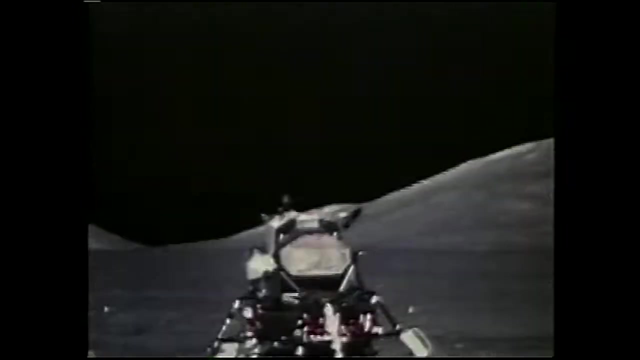 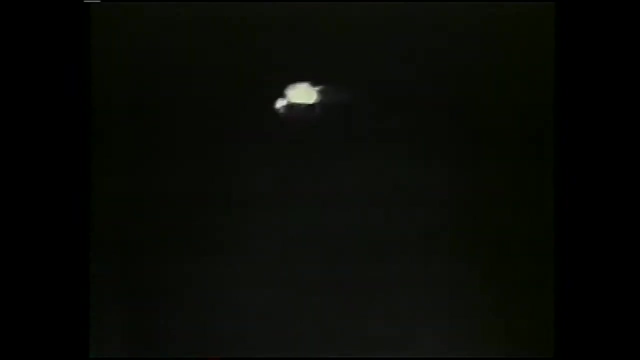 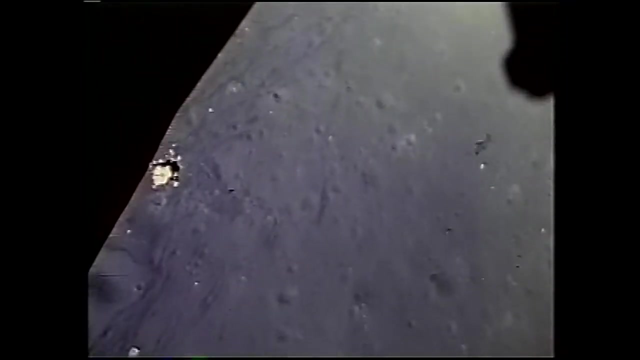 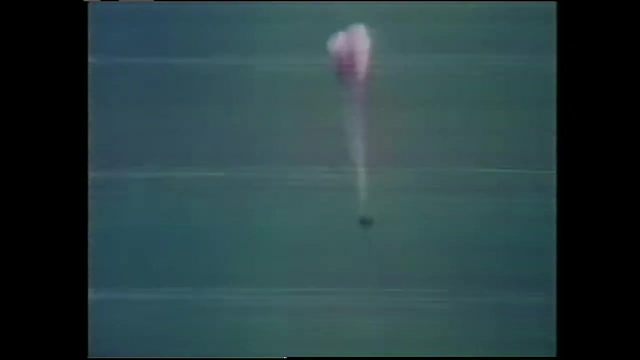 You'll do the same thing. You see, When you walk on the moon, you can change your mind. And here they go, blasting off from the moon to go back to Earth. Hey, they can see their shadow on the moon. Look at those parachutes. 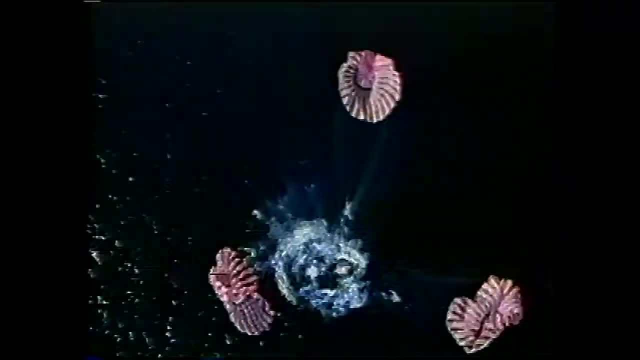 And now they're back home safe and sound. And here they go, blasting off from the moon to go back to Earth. And here they go, blasting off from the moon to go back to Earth. Hey, Hello, Mike, Welcome to the Kennedy Space Center. 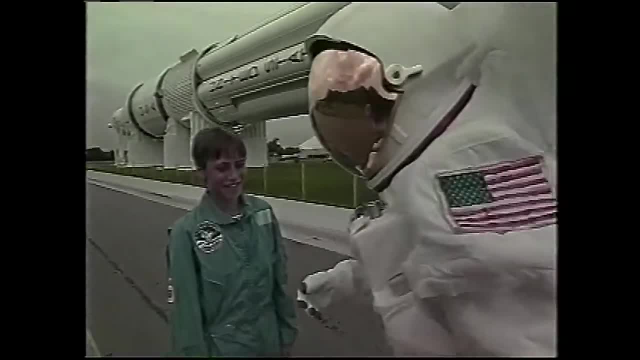 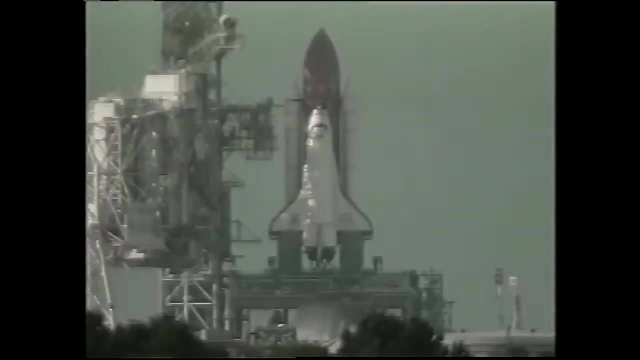 So, uh, you're an astronaut from a space shuttle, right? You bet This is a suit, just like what they wear when they go to work in the cargo bay. Hey, let's watch a space shuttle launch D-10,, 9,, 8,, 7, 6.. 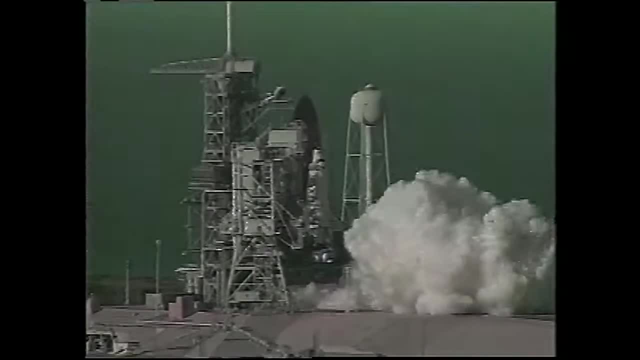 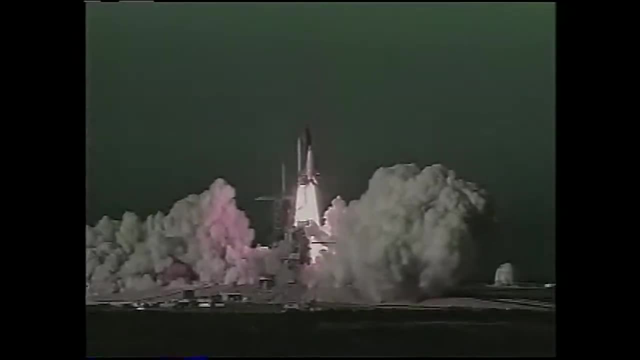 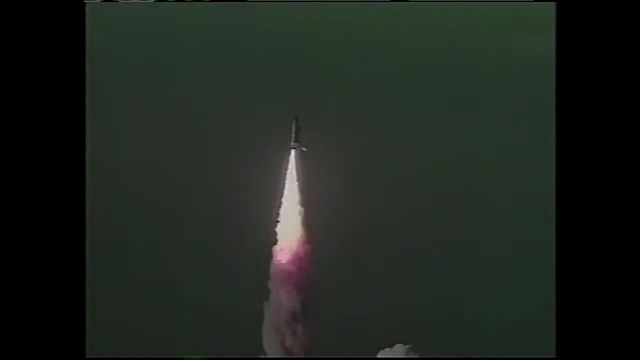 Main engine start Three engines up and burning Two. one Liftoff. Liftoff of space shuttle Discovery developing new techniques to monitor our Earth's environment from space. And this is the payload bay for a shuttle. It's where all the cargo goes. 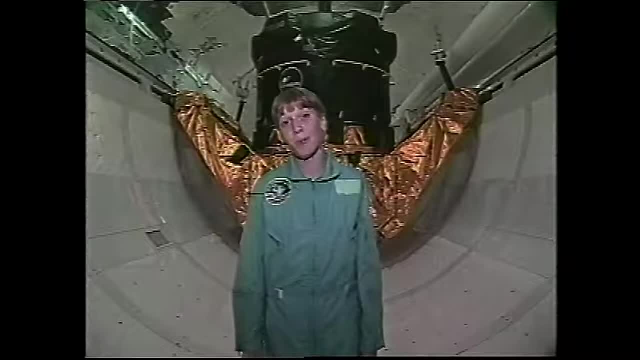 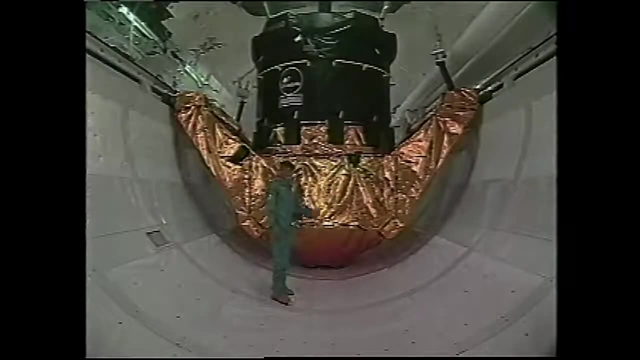 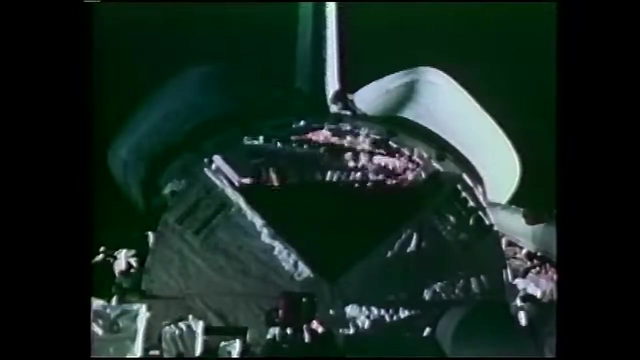 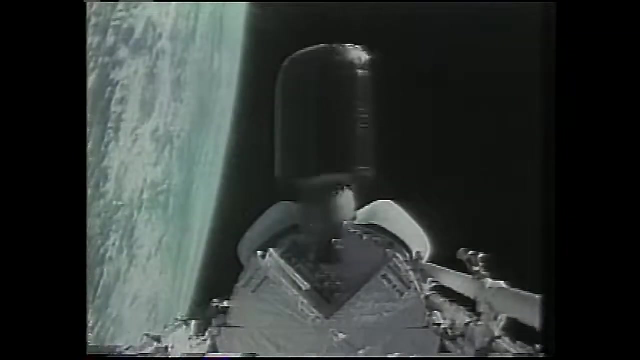 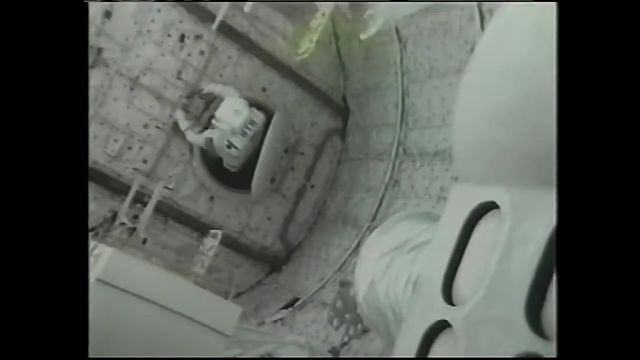 Because a space shuttle can haul so much stuff up into orbit. some people call it a space truck And this is a satellite which gets launched up into space from the shuttle, space from the shuttle. 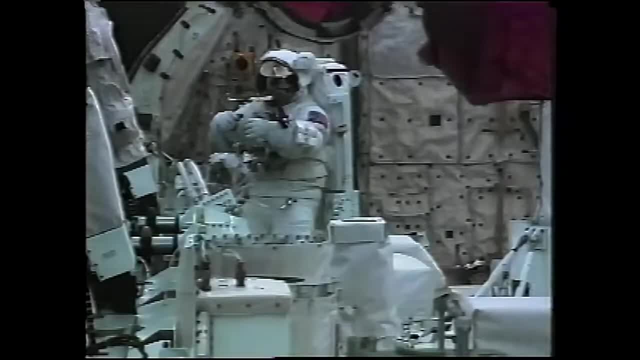 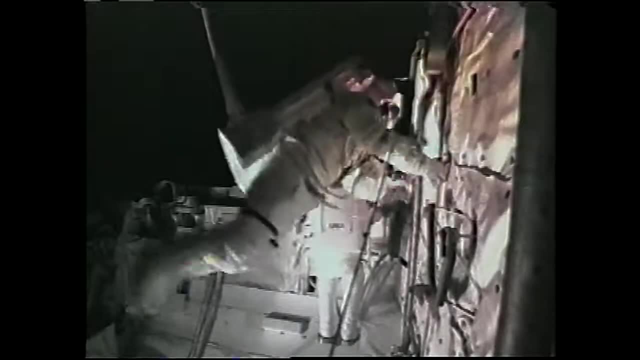 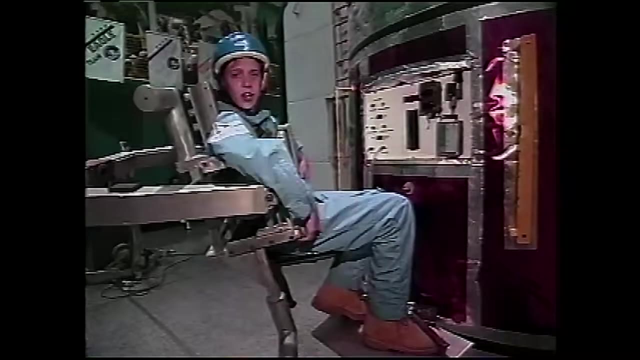 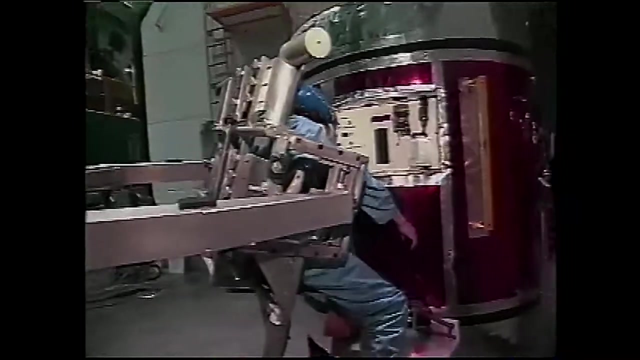 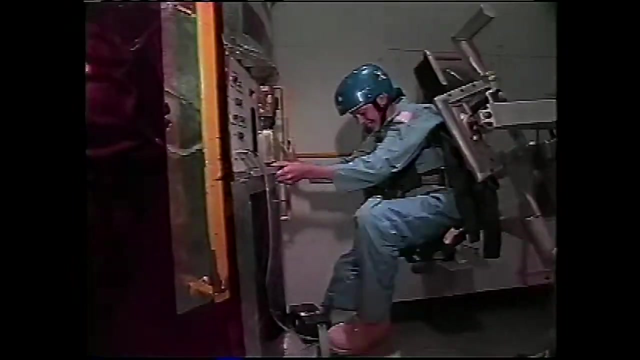 This machine is called the five degrees of freedom. It simulates what it's like to walk in space. Now I'm going to do something I might do if I were in space. 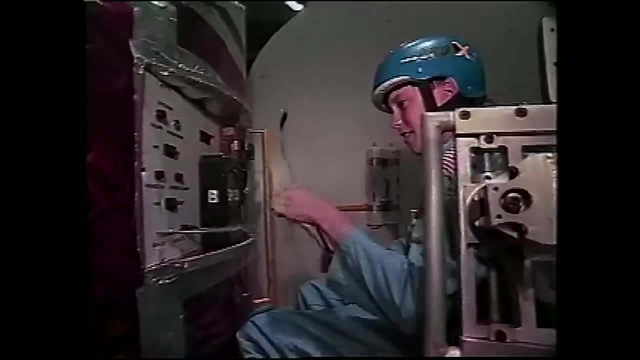 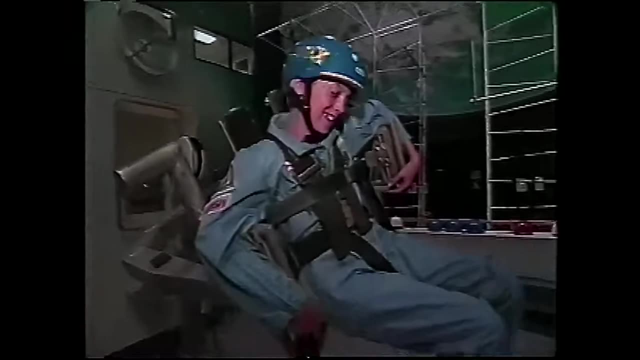 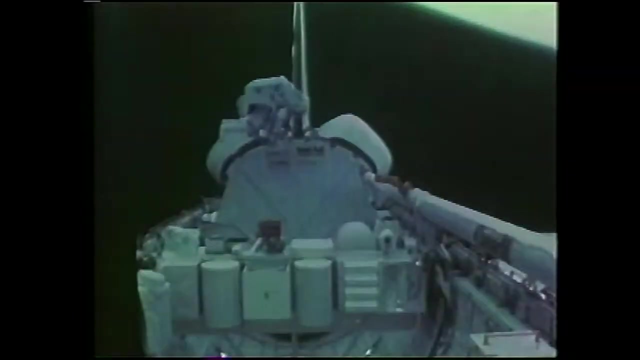 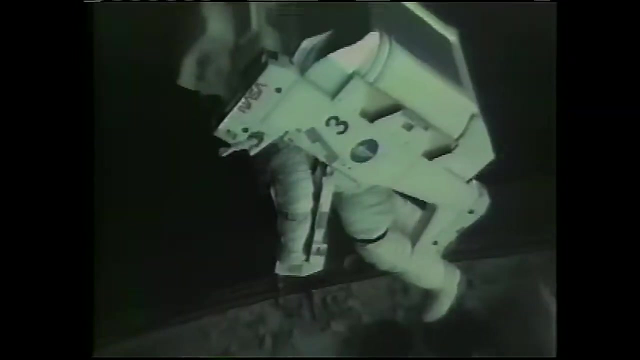 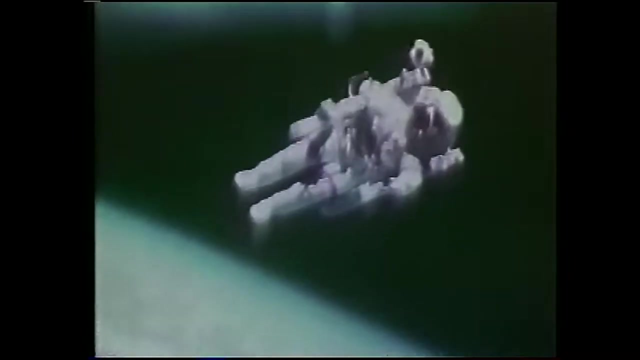 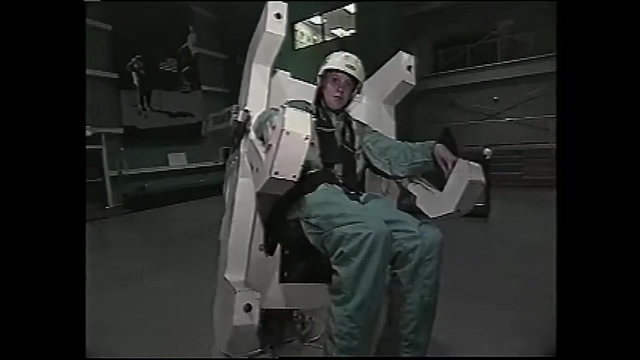 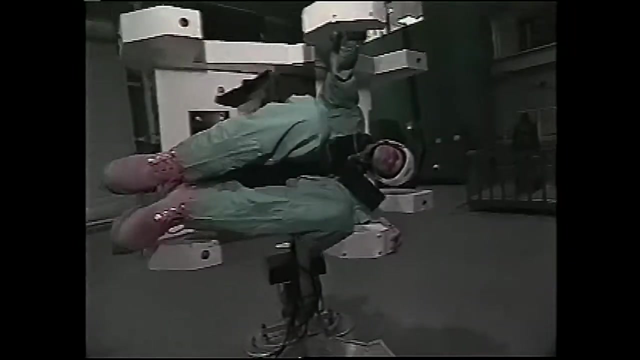 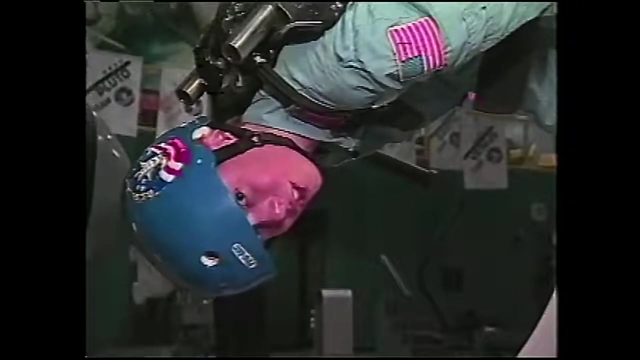 I feel like I'm just free floating. Those jet packs are called MMUs. They help the astronaut move around in space. 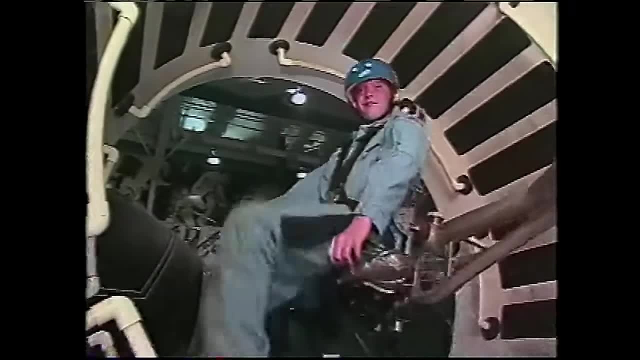 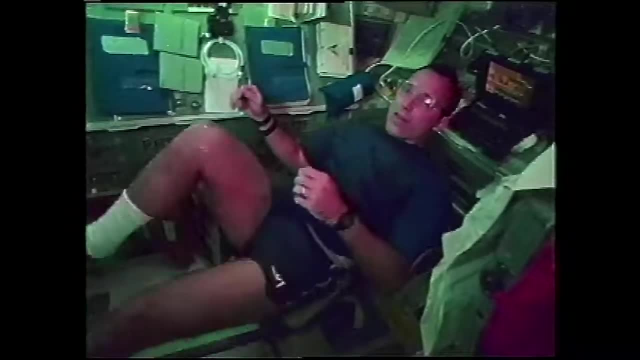 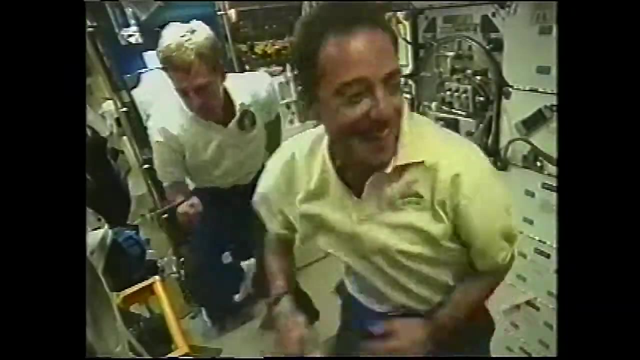 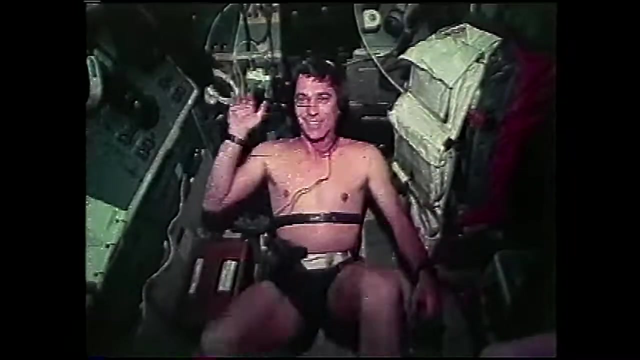 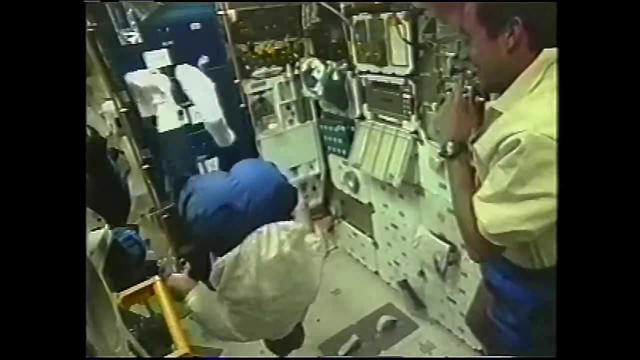 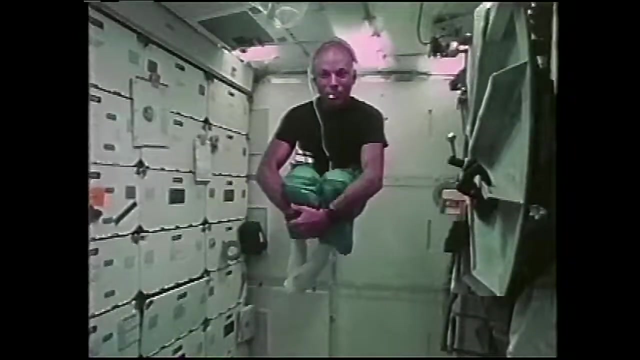 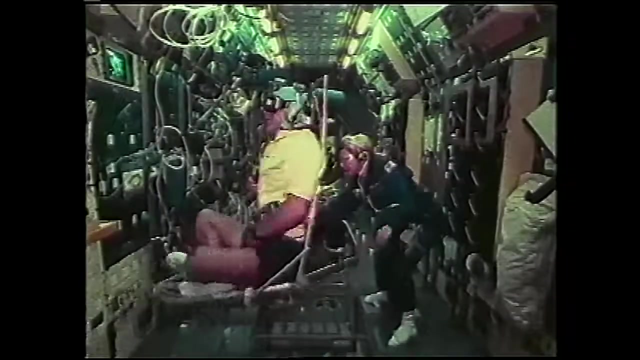 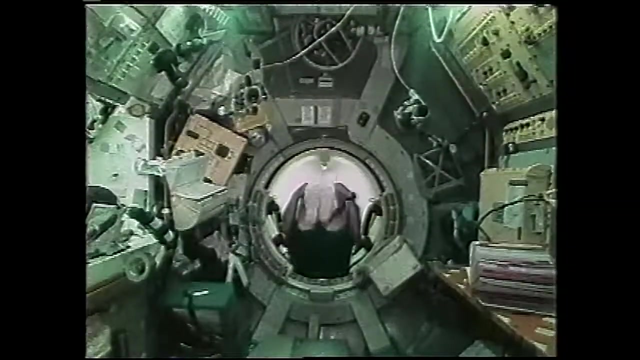 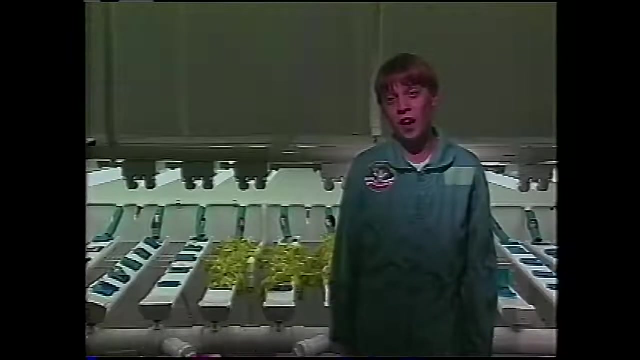 guitar solo In a space station. astronauts will have to grow their own food. They'll grow them hydroponically, which means they'll grow them in water. Astronauts sometimes eat freeze-dried food, such as this freeze-dried peach. 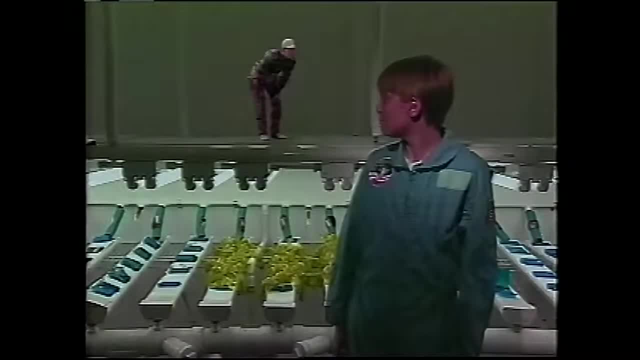 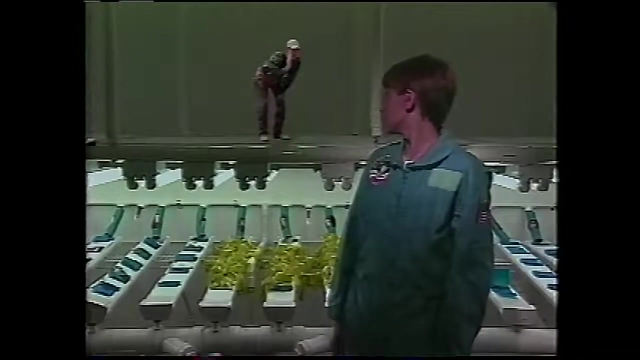 Mmm, Pretty good, Hey Pop. it seems like those astronauts do a lot of work, Don't they get any time off? Well, they do eat and sleep, of course, Hey, but then they are weightless, so they do goof around. 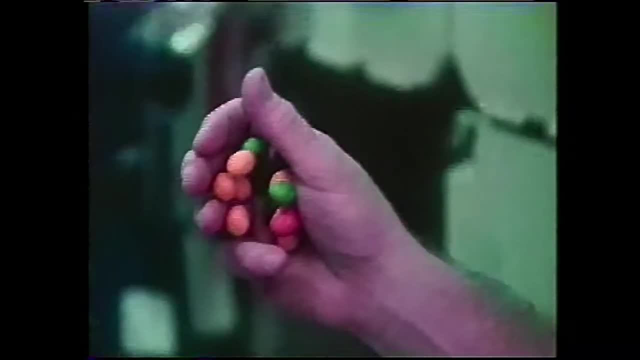 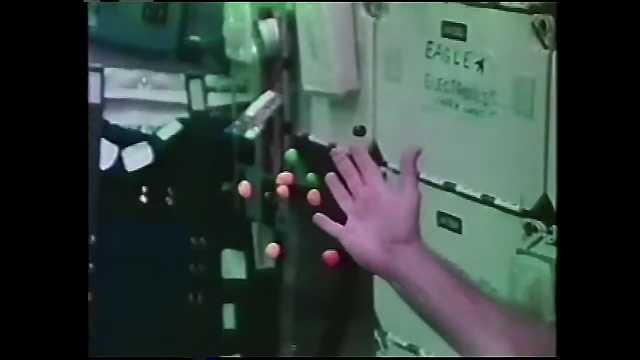 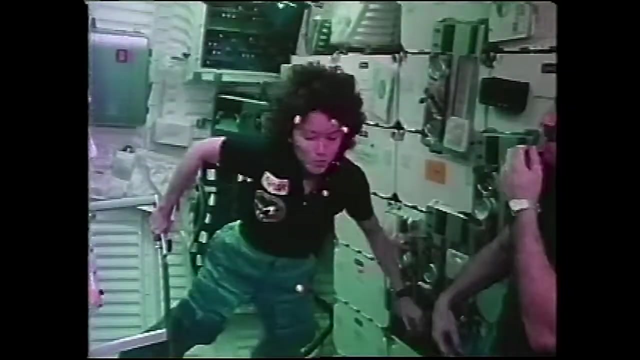 They do goof off a little bit too. Are those M&M's? Yep, Wow, M&M's in space. Bet you can't eat just one. How many are there, Mike? Eight One, Seven. See, I told you she couldn't eat just one. 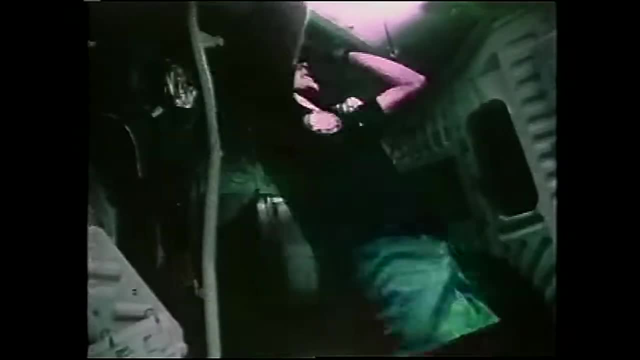 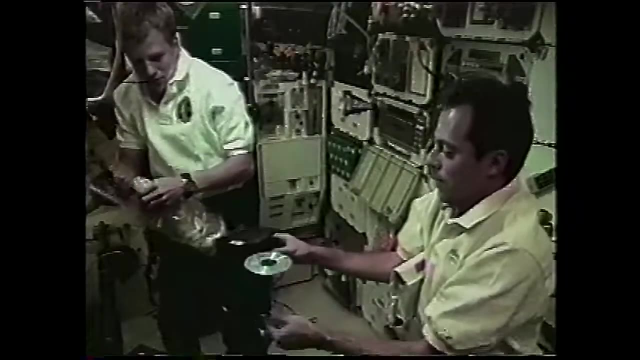 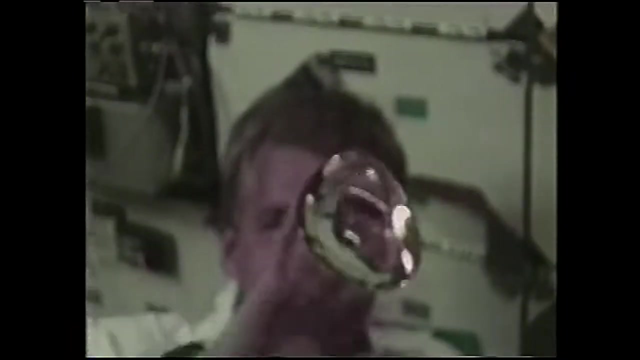 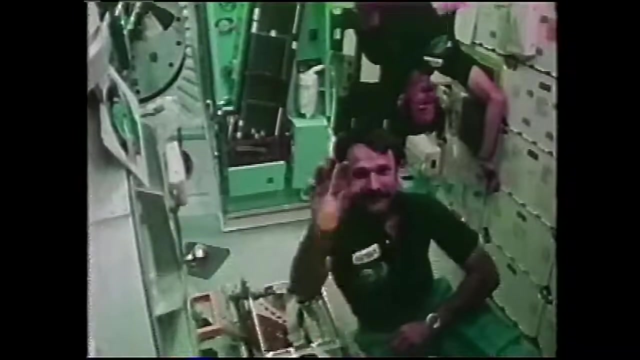 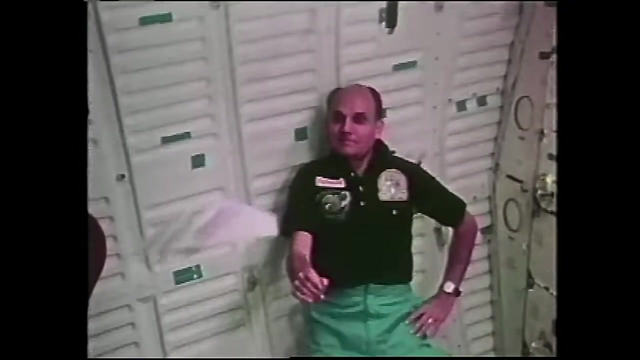 One, Two, Three, Oh yeah, Oh yeah, Three, Four, Let's go. Oh yeah, So I'm going to grab the face, the little golden "DHM" and throw every last one at the windpipe testing machine. 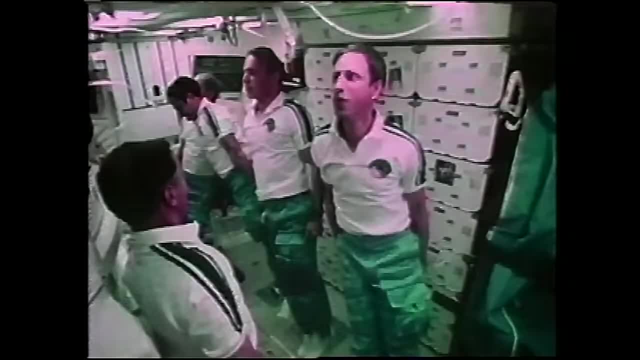 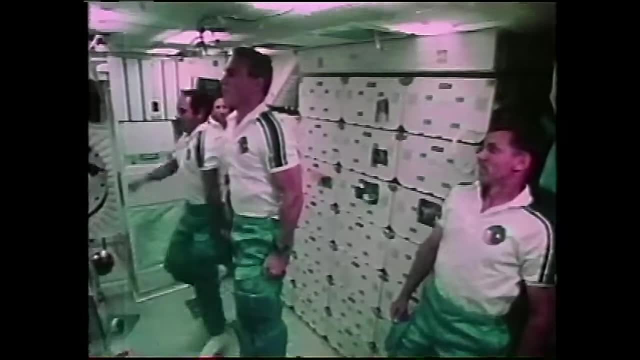 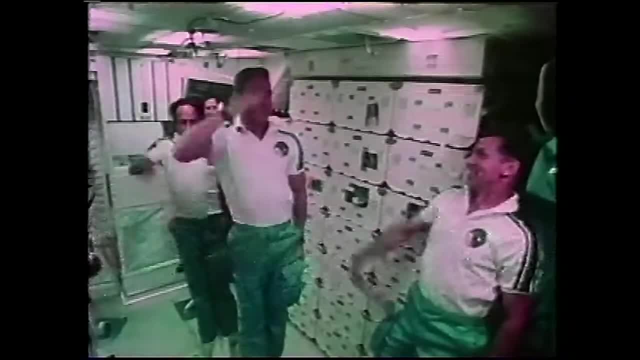 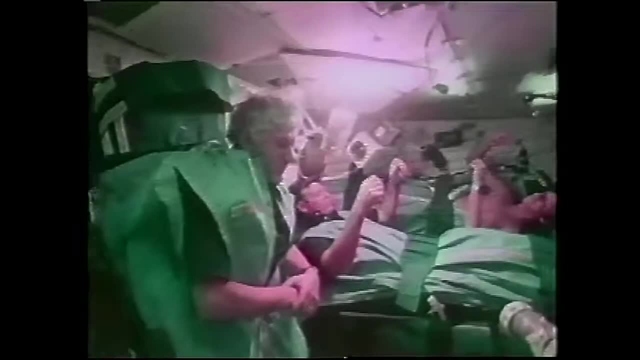 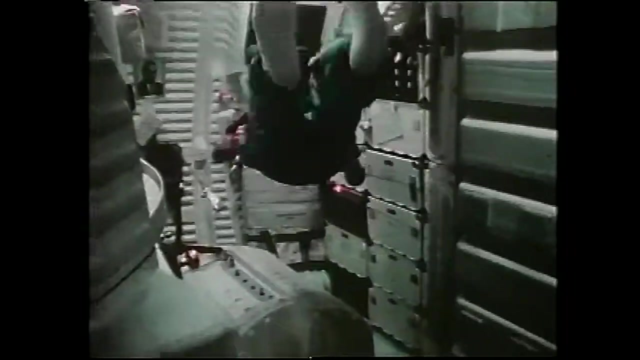 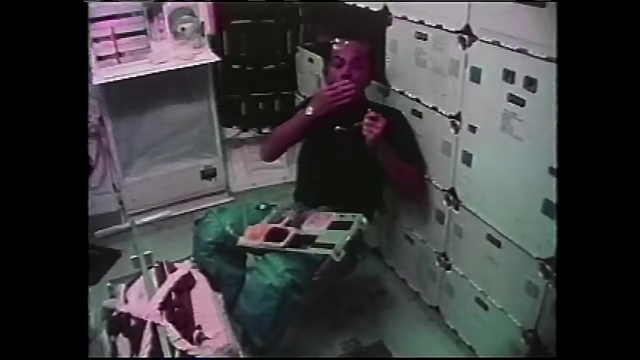 One, two, three, four, stop. Thank you, sir. Look their arms flow when they sleep. How would you like to get your pants on like that? Mike Whoa, their food floats when they eat Pop. that settles it. 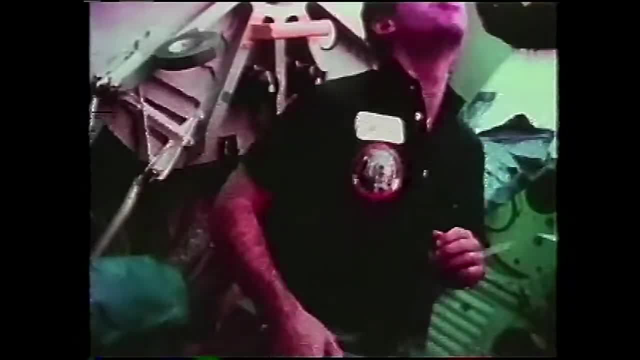 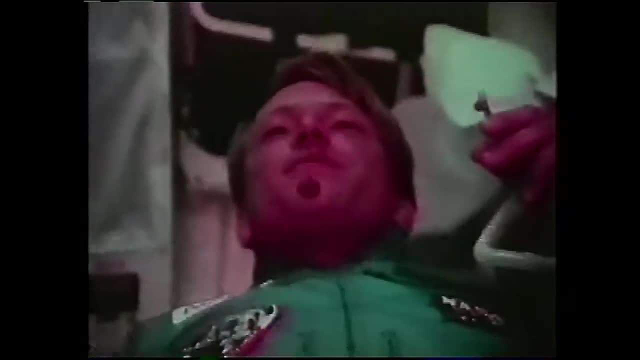 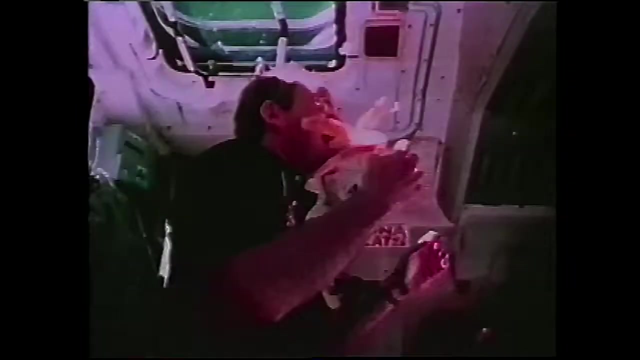 When I grow up, I am definitely going to be an astronaut. When I grow up, I want to be an astronaut too. Pop, you are grown up. Oh yeah, I forgot. All right, Catch that banana. Ha ha ha. 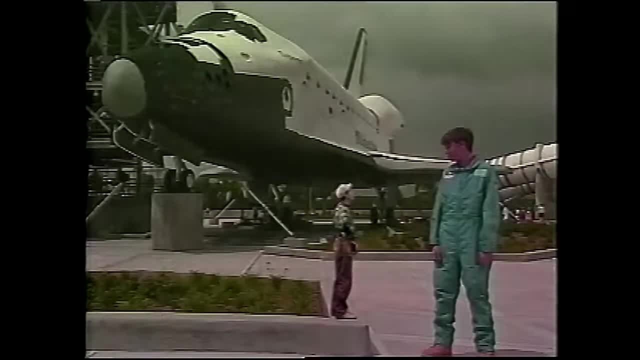 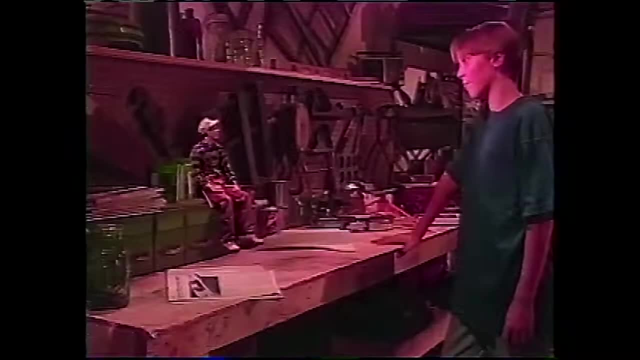 I'd like to eat your dessert like that Pop. I think our mission is completed here at Kennedy Space Center. Excellent job, Mike. That was great at space camp. Pop, Thanks for the trip. You're welcome. Hey, you ready to build your shuttle now? 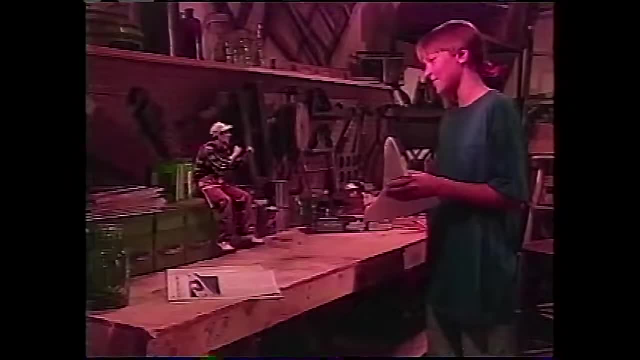 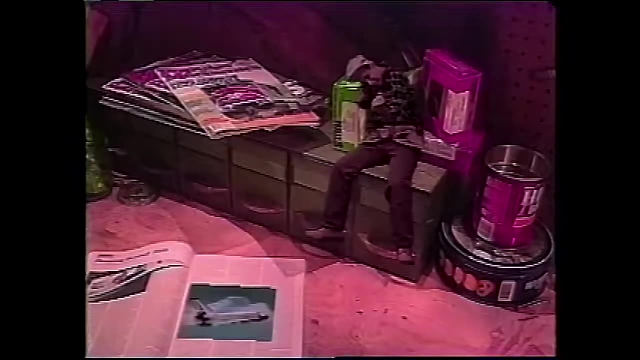 I could do it blindfolded. Great, because I got an idea. After it's finished, I'll get in the payload bay, Then you go up on the roof with your biggest slingshot And then you can send me flying.